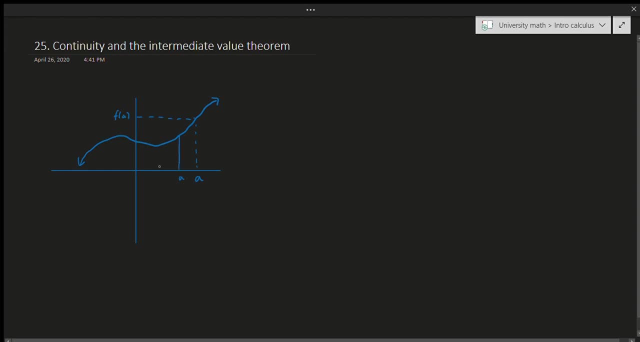 value could be anywhere. There's an e value here. There's an e value here. There's an e value here. Regardless of where I pick a as my value, there's no break points, So there's no holes or jumps or asymptotes or anything weird like that going on. 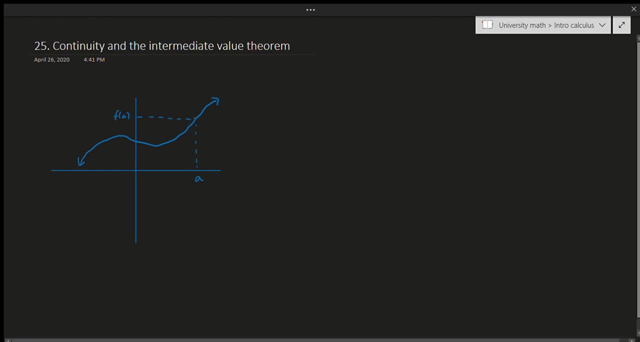 So that's what it means for a function to be continuous. There's a more formal definition: A function is said to be continuous at a point a if the limit as x approaches a point of a function is equal to the value of that function. So what does that mean? So let's do a bit more of a. 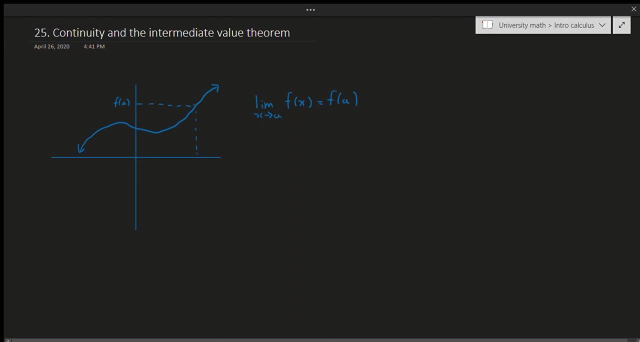 concrete example, just to kind of demonstrate what it means for a function to be continuous. So let's go right at it. So let's scroll down a little bit, Okay. So let's see, Let's draw another axis, Okay. So suppose I have this graph right here, So let me use a different color for this. 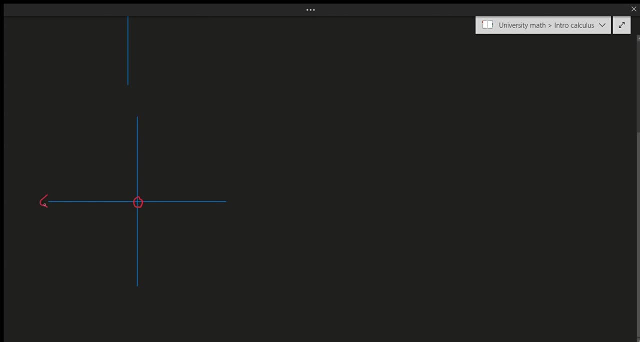 So here's an open dot here, And then this is a line that goes to the left, And then there's another line, This one is closed, And then this one is closed, And then this one is closed, And this one goes this way. Okay, So suppose that this point right. there is the value of 1.0.. So the 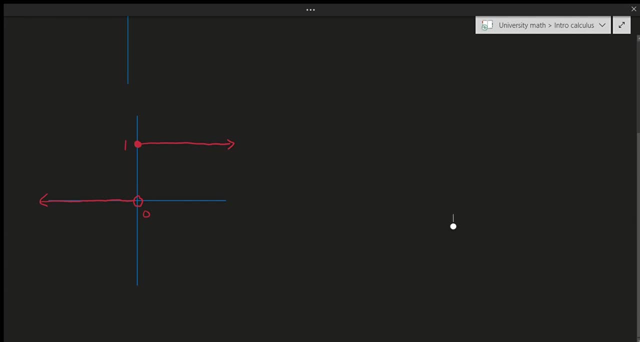 y value, just to be clear. So this is known as the Heaviside function, or sometimes it's called the switch function. It's a very useful application used in electrical engineering to demonstrate how to kind of represent on and off. But I mean, I'm getting off topic here. So, that being said, 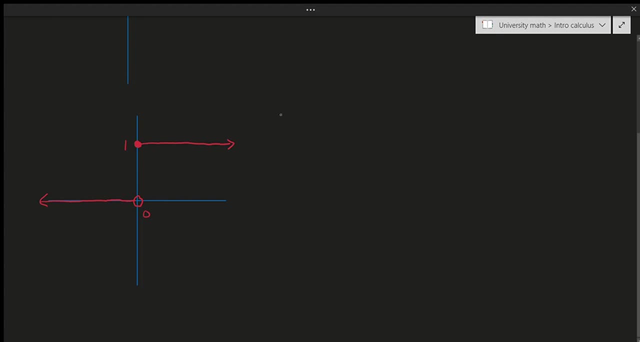 let's write down the definition of this. So in this case, h of t, which is so. h is, as I mentioned earlier, h is called the Heaviside function, But regardless, I'm just saying a function, h of t. So in this situation, it's 0 when t is less than 0.. And it's 1 when t is. 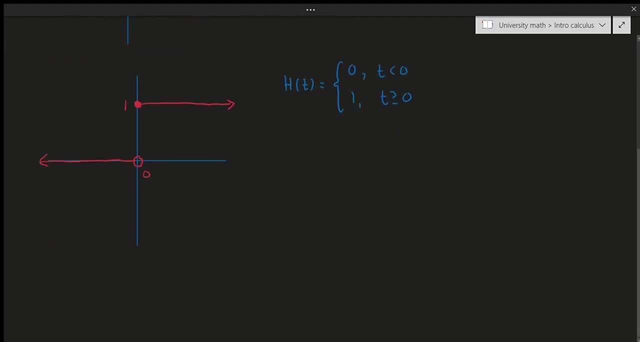 bigger than or equal to 0.. Okay, So is this continuous everywhere? No, it's not. And the reason it's not continuous is because if I take the limit as so, that's a really bad m. So if I take the limit as not, x t approaches 0 from the left of h of t. 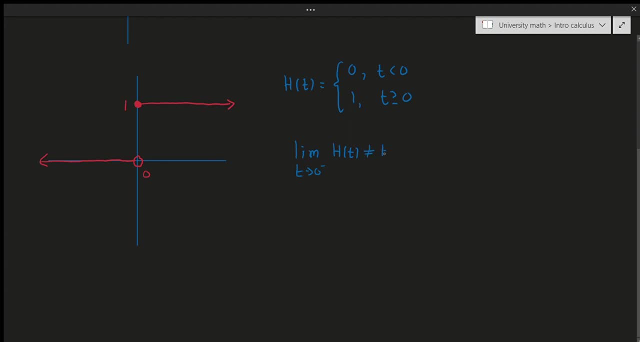 this is not equal to h of 0. And the reason for that is because the limit as t approaches 0. from the left that's 0.. So 0.. And the value of h of 0, according to this definition, is 1.. And 0 does not equal 1.. So the function is not continuous. 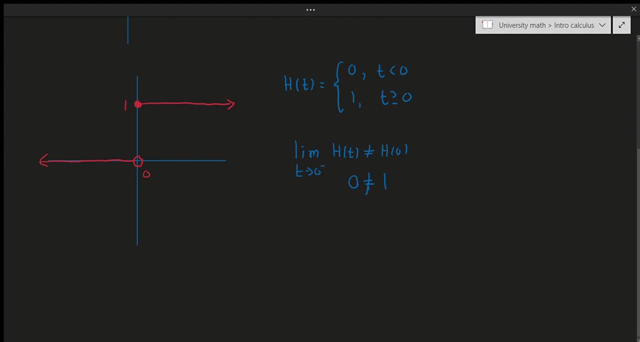 across its entire interval. So, for example, here in this kind of arbitrary graph, it was continuous, because I could take the limit across all points regardless of direction, and I would get the same value. Another kind of a shortcut of saying this is: I should be able to draw the graph without 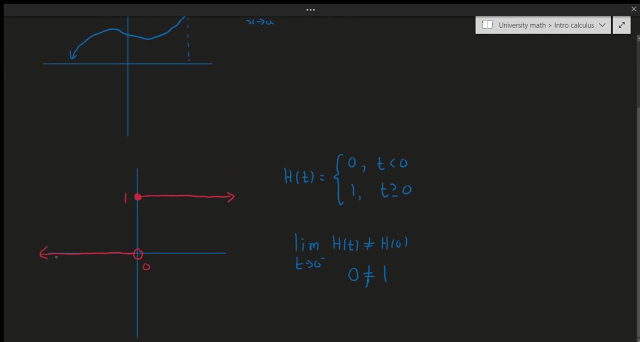 ever kicking off my finger. So right here I can draw a graph, that's fine. But here I have to take off my finger, go up here and continue here. So if I have to do that, the function isn't continuous. So that's kind of a quick and dirty way of doing. 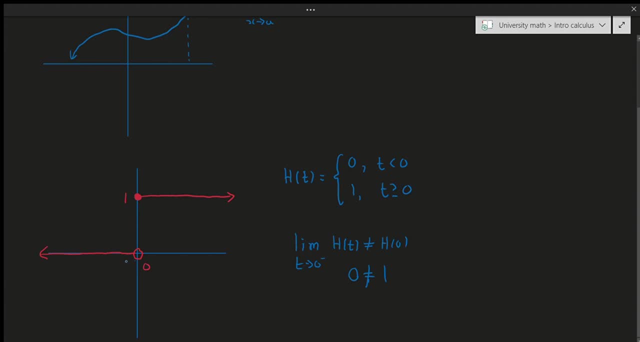 that Okay, so let's keep going. So these are all sort of equivalent statements for a function to be continuous, So let's write them down. So some properties, So some properties of continuity. so let's go ahead and underline that, just to be really clear. 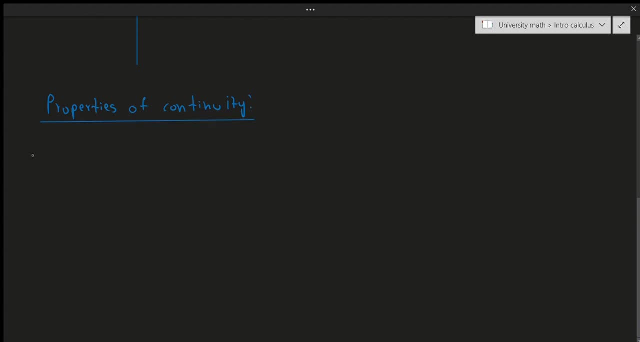 okay. so the first property, as we already talked about, is that the limit as x approaches a of f of x must equal the value at that point, okay. the next one is just kind of straightforward. this one is just saying the limit as x approaches a from the left of f of x must equal the function. 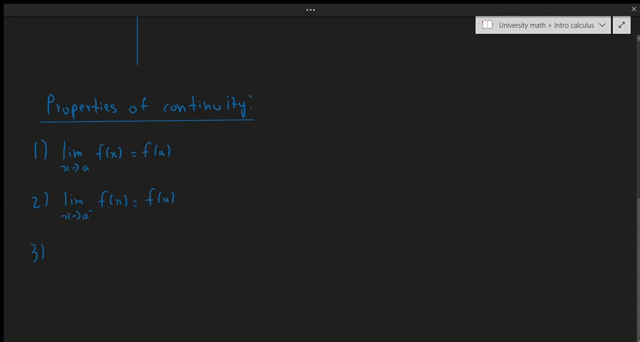 at that point. i mean that's kind of obvious. it's the same thing, the same thing with the other one. as you can probably guess, the limit as x approaches a from the right of f of x, that also has to equal f of a. so it's kind of same idea here. so what i'm getting at is that, regardless of the direction, 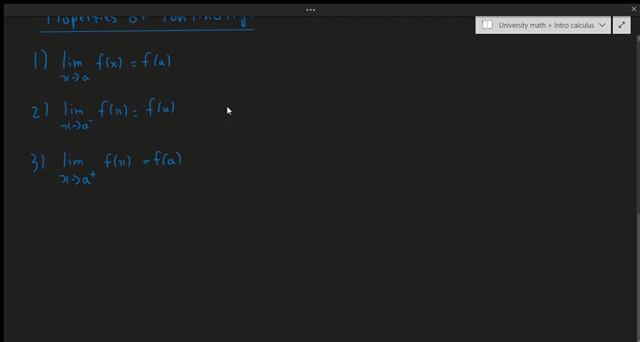 which you approach from. they all have equal f of a constantly. consequently, we can also write this down: the limit as x approaches a from the left of f of x must equal the limit as x approaches a from the right of f of x. so this is probably the most. 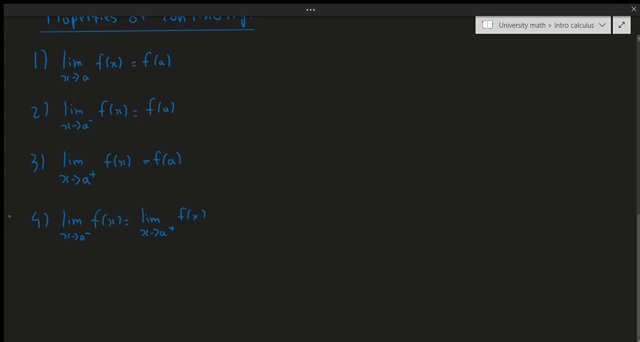 useful property, but regardless, they're all kind of saying the same thing. all i'm saying here once again is that the direction in which you approach the limit from it doesn't matter. they all have to be the same regardless. so let's do a quick kind of example, just demonstrate the idea of continuity. 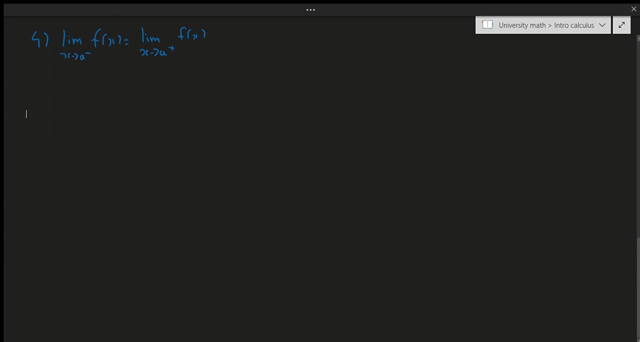 and let's see here: yeah, okay, so let's do this really quick example. uh, so let's go and do this in green, i suppose. so suppose i have this graph that looks like this, okay, and suppose i also have this graph, and i have this graph that looks like this. 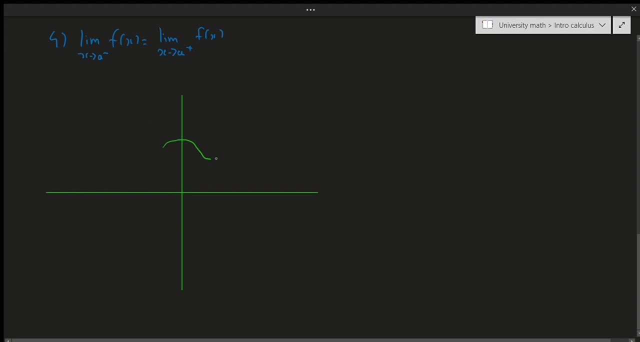 okay, and suppose i also have this graph that looks like this, that kind of looks, so it's kind of like this: so there's an open dot there goes down and then kind of looks like that. then let's see, here, this could be a little bit of an open dot there. 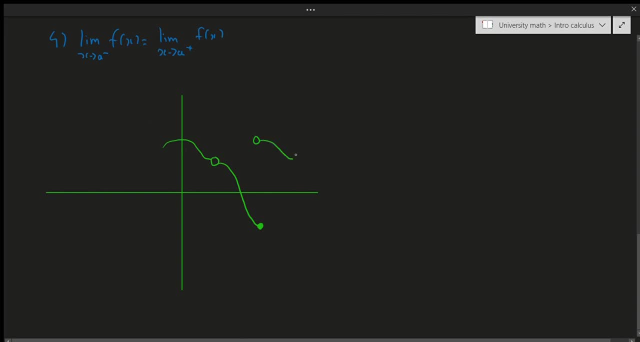 goes down- there's an open dot there- and then goes up, okay, so let's go ahead and plot these a little bit. so that's gonna be. let's say that's a one, let's say that's two, suppose that's 3, let's see. let's call that point 4, let's say that's 5, and let's see. 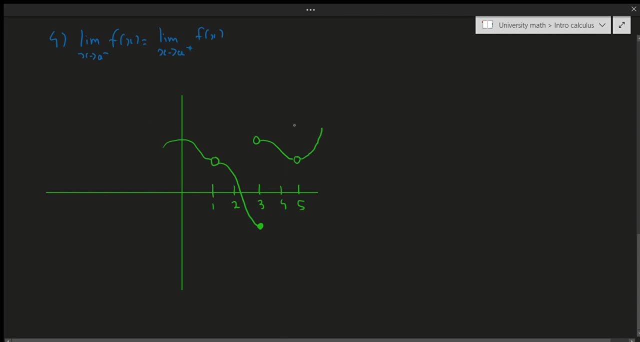 let's call this point f of 5, right there. so this closed kind of dot is denoted as f of 5, let's see, let's call this point right there, this open dot. let's call that f of 1, and let's. 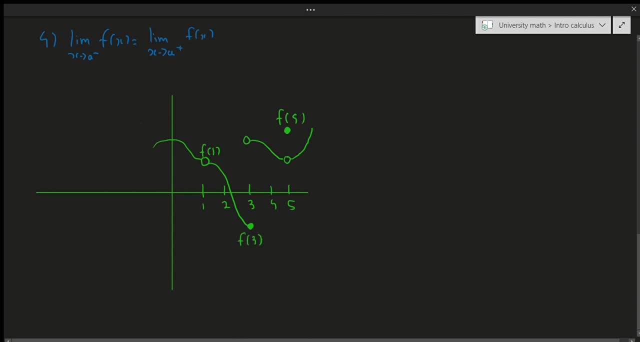 finally, let's call this point right there at the bottom. let's call that f of 3, so that's so, there, there, there and there. so let's call this y. let's call that x. okay, so let's see here. 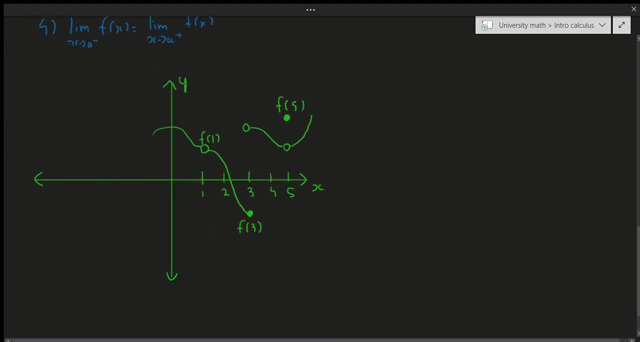 okay, so let's go ahead and do a few kind of taught examples, just kind of get you in the swing of things. so x equals 1, so does f of 1 equal the limit as x approaches 1 of f of x. so in other words, does 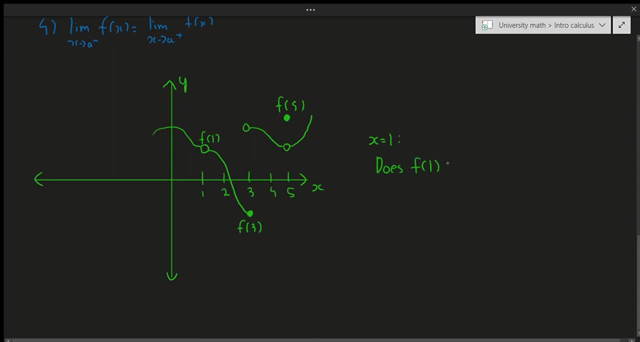 f of 1 equal the limit as x approaches 1 of f of x? well, no, it doesn't, and the reason for that is because f of 1 is not even defined at 1, there's an open dot there. so 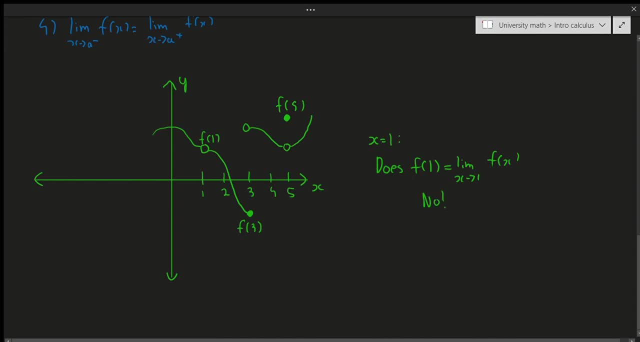 so no, so that's fine. so if it's not even defined at 1, then you know it's not continuous. okay, next one. so let's suppose we have x equals 3 now. so does so, just to be consistent, does? 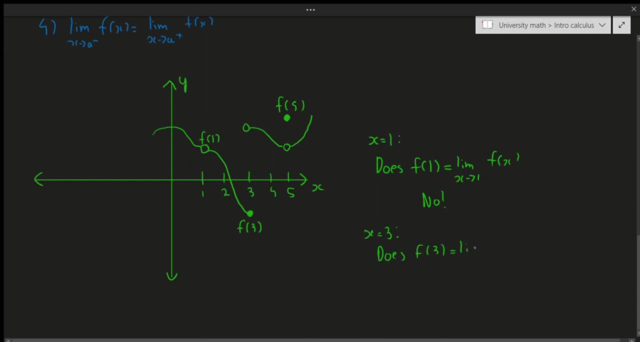 f of 3 equal. the limit as x approaches 3 of f of x. well, okay, f of 3 in this situation is equal to right there. and then the limit as x approaches 3 of f of x. well, that doesn't actually exist because as you approach from the left. so let me. 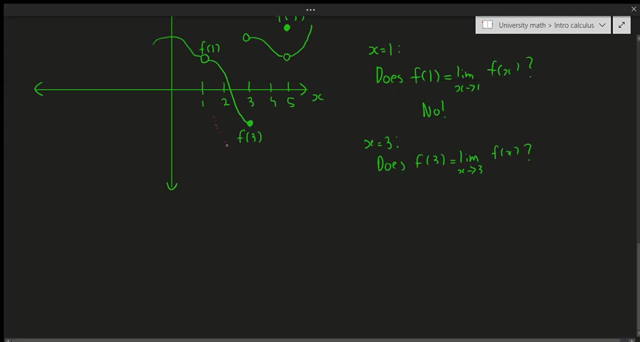 use a different color for this. as I approach x equals 3 from the left, I get this bottom value. but as I approach x equals 3 from the right, I get this top value. so the limit doesn't actually exist. so 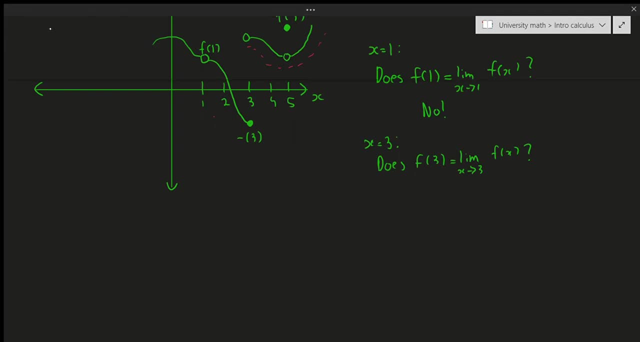 that's. that's not good. so as a result, that's also not continuous, so let me just kind of undo that eraser by accident. yeah, so let's go ahead and fix that a little bit. there we go, okay. so does the function equal the limit? no, f of 3 exists, but the limit doesn't. 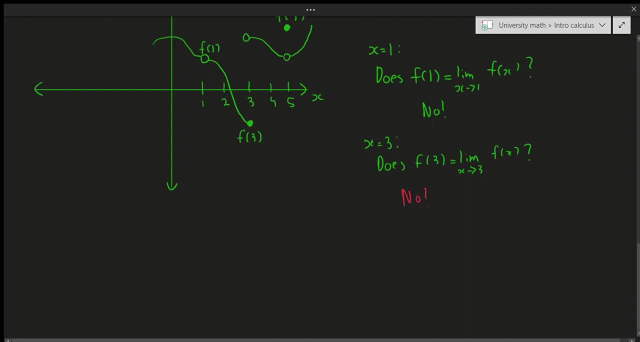 exist. so no, I'm actually going to write that in red as well. so no, so, so. so in the first one, f of 3, not defined, and in this situation the limit doesn't exist. okay, what about the next one? so in this situation, we have: x equals 5,. 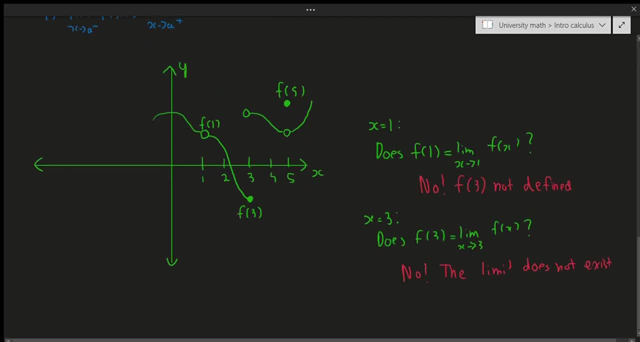 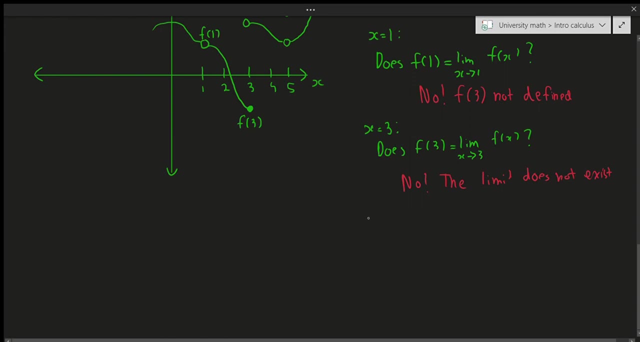 well, the problem with this one is that at x equals 5, so let me just actually write that down, just to be consistent with everything. so at x equals 5, so does f of 5 equal the limit as x approaches 5 of f of x? 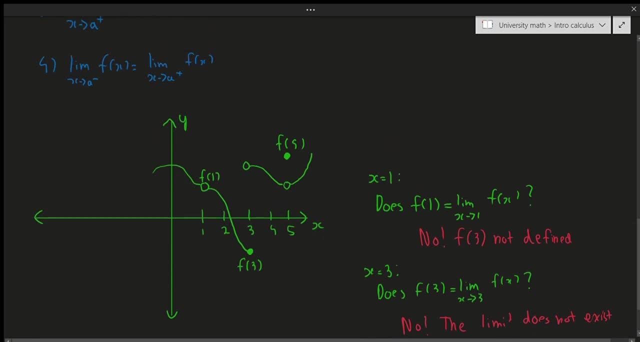 well, that's certainly not. that's not true. f of 5 is up here, but the limit as x approaches 5 from both directions. is this point right there? so the limit does not equal the y value. so no, that's not true. 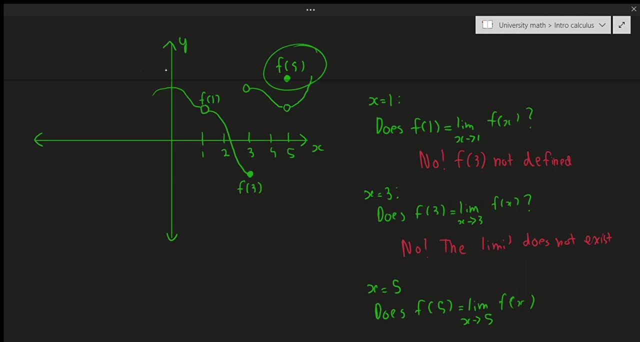 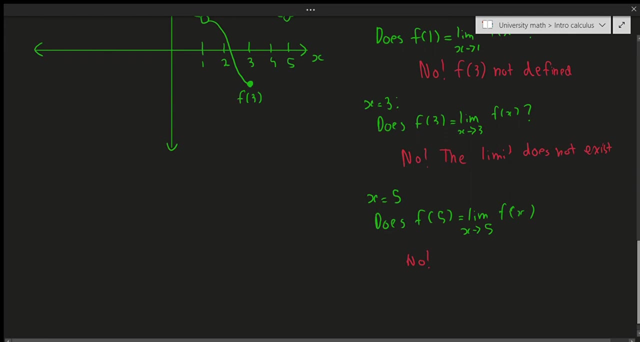 so no, f of 5 does not equal the limit, because there's different y values. the limit equals this point, but the y value is up here, so that's not true. okay, so as a result, none of these, none of these. it's not continuous across any of these. 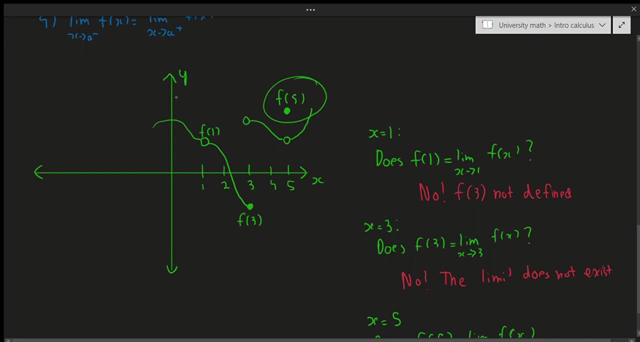 points it might be continuous over like a small interval, like, for example, that's certainly continuous, and like this section is continuous, but this over its entire domain. it's not continuous because, for example, once again, if I draw, 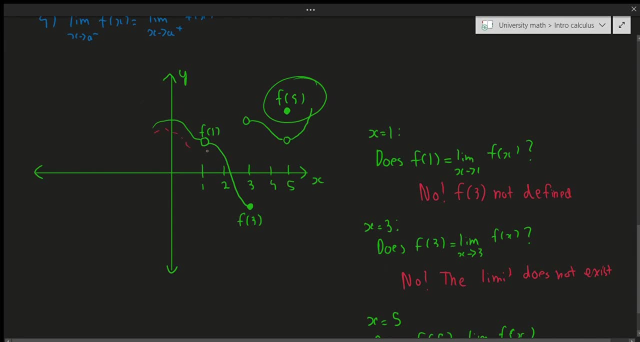 this graph. I have to take off my pencil up here, continue, and then take off my pencil again here, continue, just take off my pencil again and then continue on. so using that definition, I can't- oops, sorry about that- using that definition, I can't possibly determine. 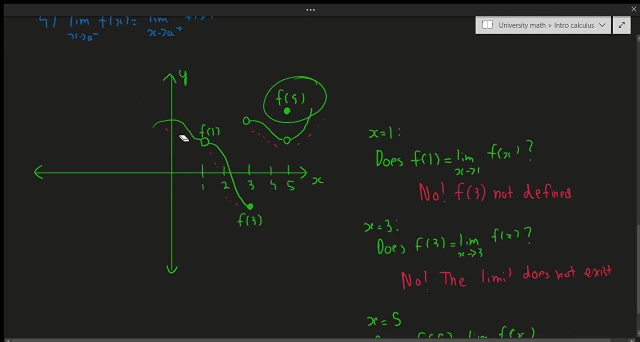 that this is a continuous function. it's not, so you gotta be very careful about that. so let me just kind of erase the red parts a little bit. there we go, okay. so there's that now. 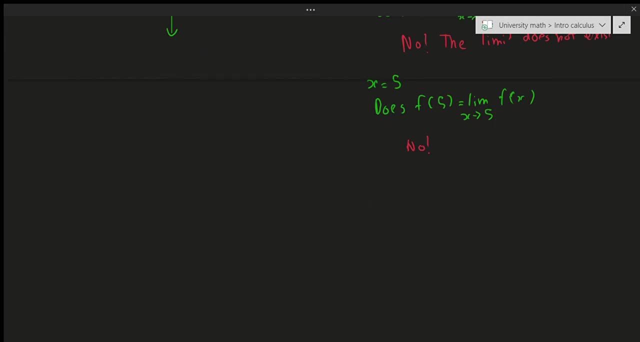 let's do another example where it, where it is continuous. so this one is a very simple example, so I'm just going to kind of do this a little bit quickly. oops, let me just draw a graph. there we go. so suppose I want the parabola: y equals x squared, so y equals x squared. 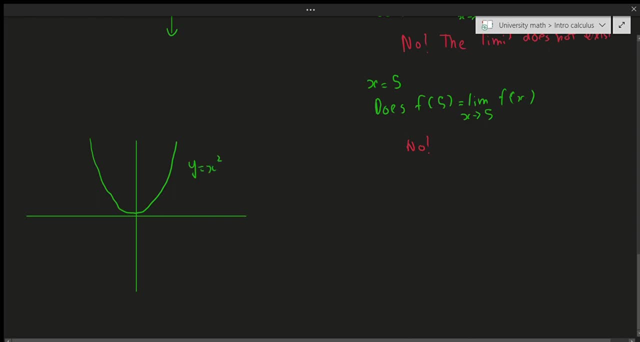 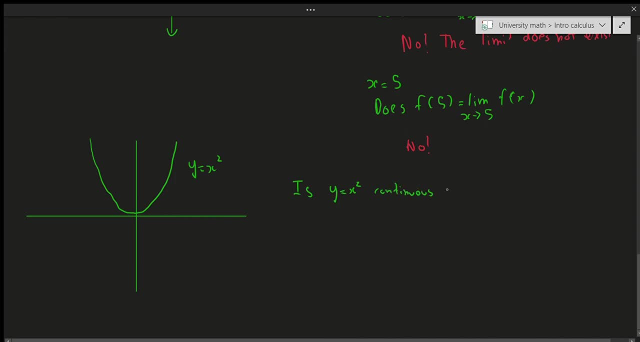 at x equals zero. yeah, it is, and the reason for that is because the limit, so let's go ahead and do this. the limit as x approaches, zero of x squared is equal to f of zero. well, what's the limit? well, that's obviously zero. 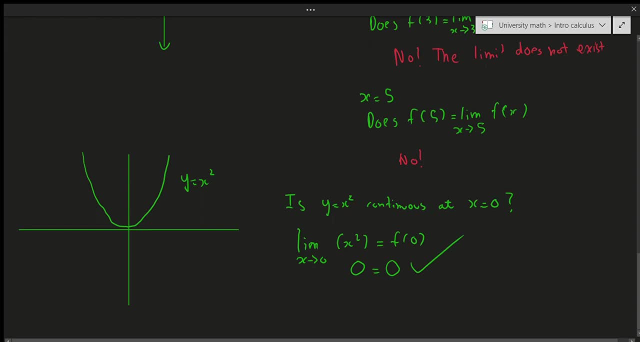 and what's f of zero? well, that's equal to zero as well, so they're equal. so, yes, it is continuous at zero. okay, so that's not too bad at all. now let's do an interesting. 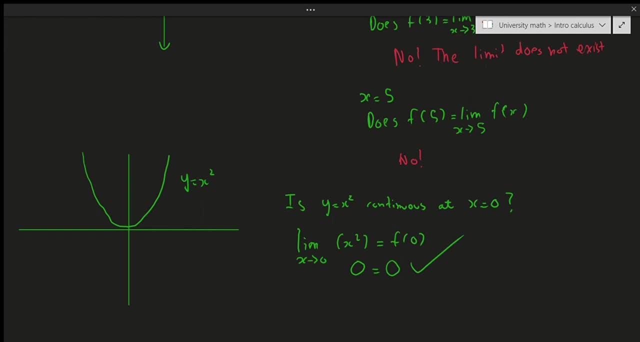 sort of example. but before we get into that example, there's a few things I need to talk about, about common kind of functions. so what do I mean by that? so the following functions are always continuous, just because, well, it's kind of obvious. if you want a proof of it, 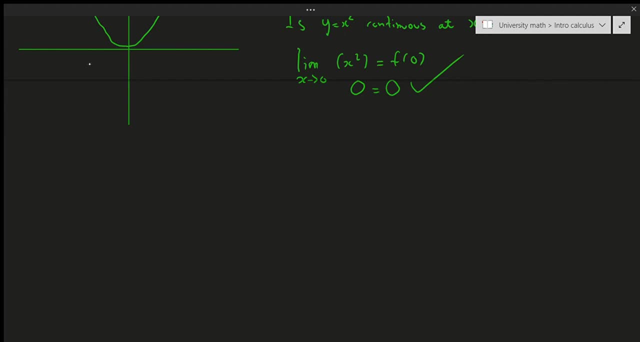 leave, leave some. leave something in the comments and I can make another video about it. but hopefully you will kind of recognize that the following kind of the following, by definition are supposed to be continuous. so some other properties. so I'm going to use white for this. 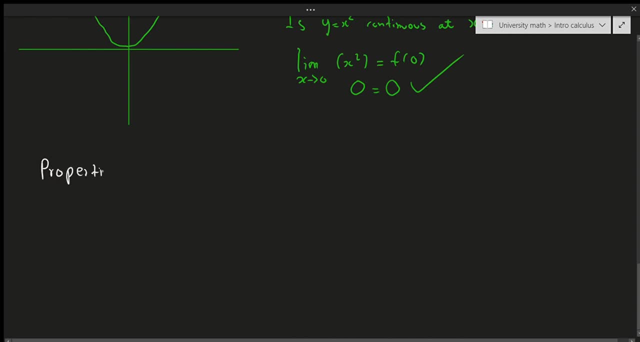 part. so properties, okay, so some very basic properties. properties: one, two, three, four, five. okay, if f of x and g of x are continuous functions, then f plus g is continuous, f minus g is continuous. 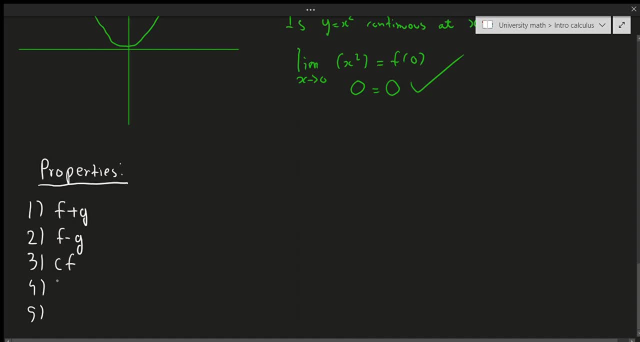 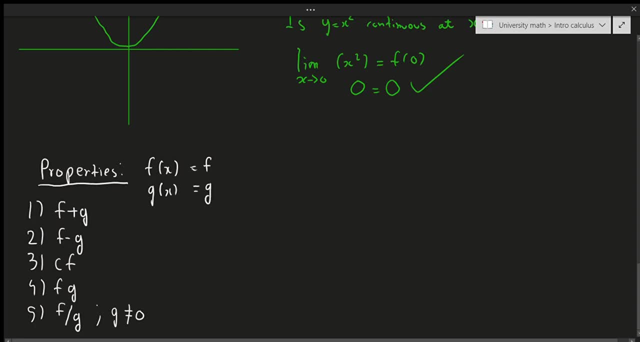 and g of x, which once again I'm going to denote it as g, if both of these are continuous functions. so if f and g are continuous, the following properties: right there they hold. so that should be fairly obvious. I mean, if I have two continuous functions and add them. 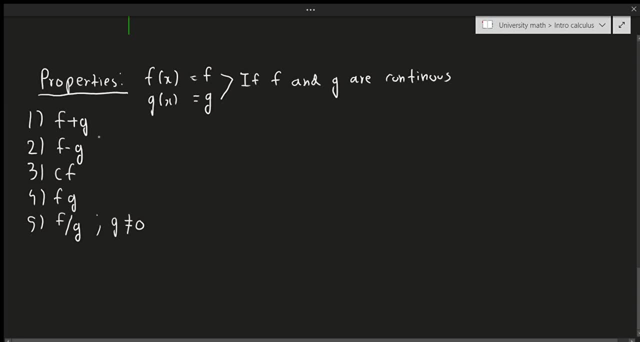 they're going to be continuous. if I take a difference of it, that's also going to be continuous scaling. a continuous function is not going to affect the function. so multiplying two continuous functions is not going to change anything. and if both functions, 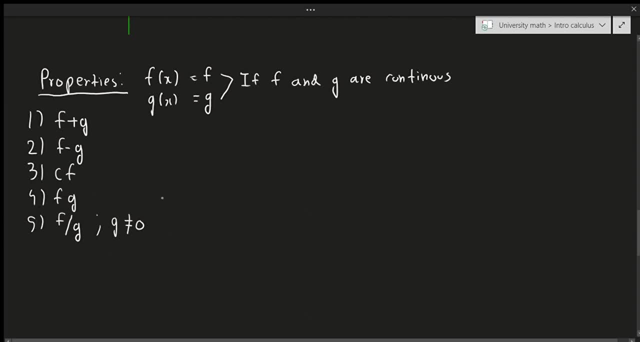 are continuous, then dividing it is also going to be continuous, usually assuming that g does not equal zero, okay. and then the next part is the types of functions are continuous. again, most of these are fairly obvious, but you have to be very careful about it, about some definitions. 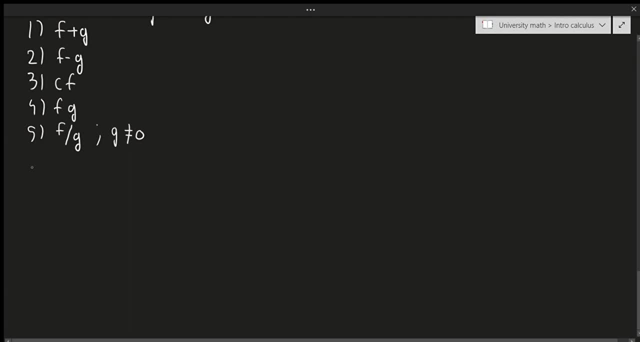 you use. so let's go to these different colors for this. so the following are always continuous. so the following are always continuous- and I'm going to write this part in red because a lot of people miss this part- the following are always continuous: over its domain: 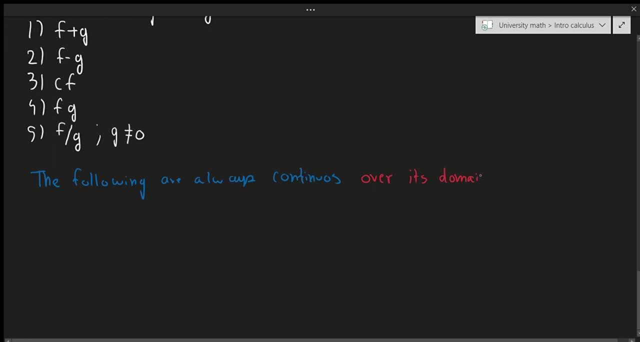 this is actually a really old exam question that was tested a while ago, back when I was taking calculus in university. the examiner put: oh, is this function continuous? a lot of people would say no, it's undefined. but the trick was that that undefined part wasn't even on its domain, so 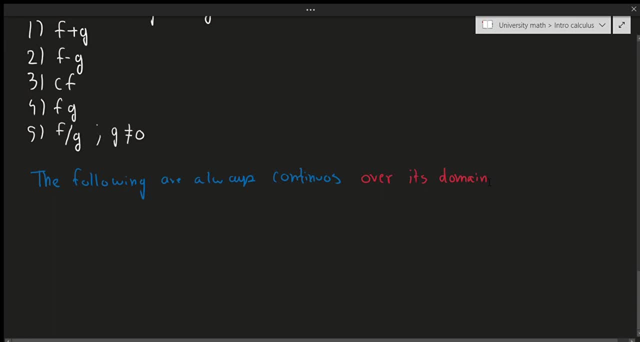 it was continuous, regardless of you know any undefined points or something. so we'll do an example of that kind of situation later if you have time, but let's just keep going. so the following are always continuous, so let's go ahead and do this. so polynomials are: 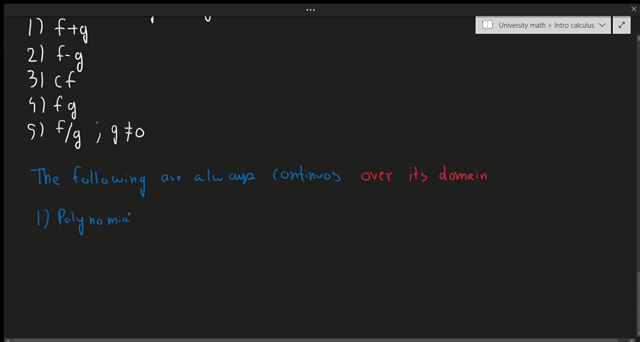 always continuous, so let's go ahead and do this. so polynomials are always continuous. this should be kind of obvious. the next one is a trigonometric function, so trig functions are always continuous. the next one is an exponential function. 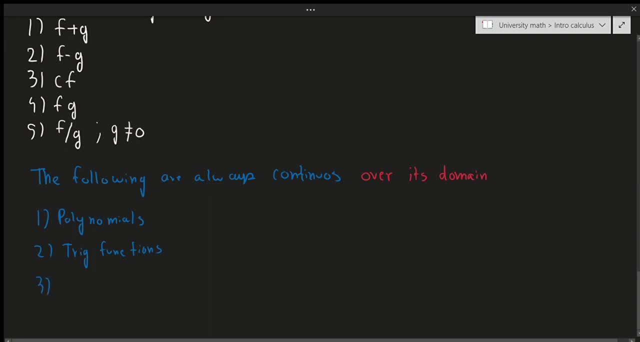 so you might be thinking, oh, but tan is undefined, it's not? I say it over its domain, so you got to be very careful over its domain. tan is most definitely continuous, so you got to be very, very careful about that. so the next one is the exponential function. 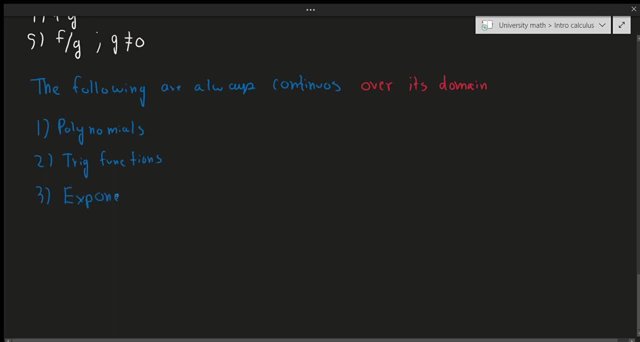 so exponential functions. that should be fairly obvious. so functions. the next one is rational functions. so rational functions. the next one is logarithmic functions. and the last one is root functions. so square root of x, square root, key root of x, things like that. 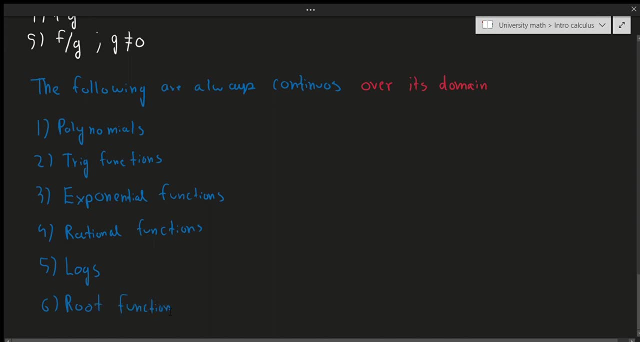 and the other thing you got to be careful about is, once again, you might be saying, oh, but the square root is undefined for all values of x less than zero. yes, that's true, but again over its domain. so, over its domain, the square root of x is continuous. so you got. 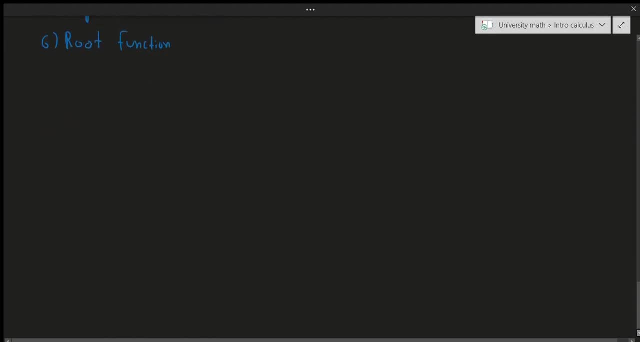 to be very careful about that. okay, so here's a very interesting question. this is actually an old exam question that was tested back when I was in university, so this will be good practice, so let's go ahead and do that. so suppose I. 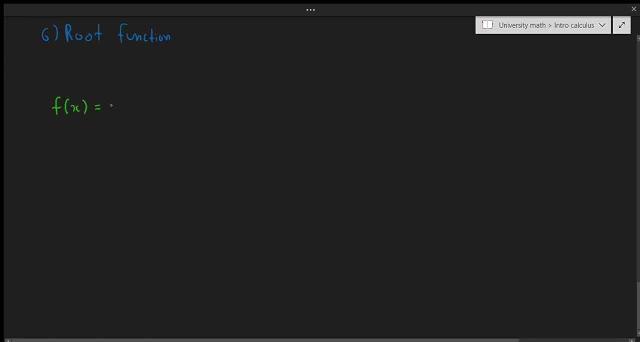 tell you that f of x is equal to. so let's go ahead and write this down. let's see: x squared plus e, x plus b. and then let's see: the second part is 2x sine of uh- wait, I just gotta check something. uh sine of pi over 2 times x. 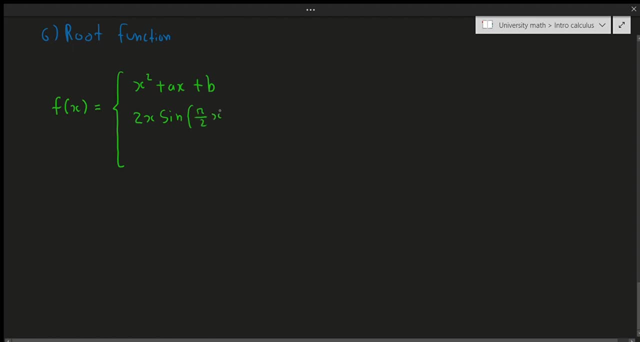 plus b, cosine of pi over 2,. uh, let's see, yep, that's good. and then let's see, we have x squared minus 4 divided by x squared minus 3x plus 2 plus e, to the 1 over 2 minus x. 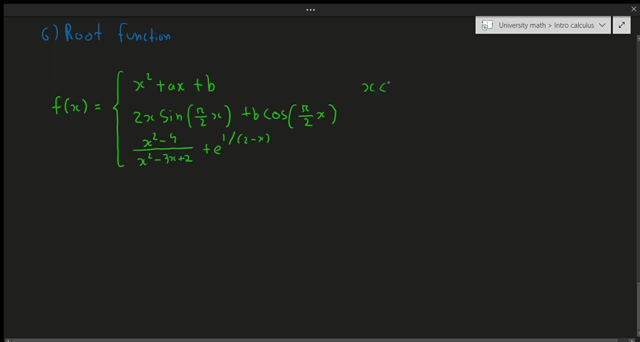 and then there's a few restrictions to this. so this one is going to be: x is less than negative 1, this one is x is between negative 1 and 2 and this one is x is bigger than 2. okay, so find. so the question was: so find all values of E and B such that 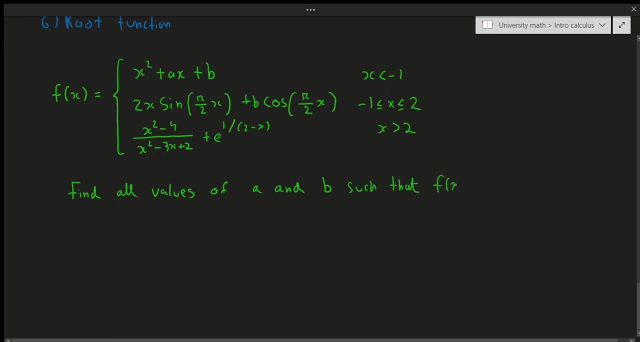 f of X is continuous. okay, so this might seem a bit weird at first, but you'll see it's actually not too bad once you get the hang of it. okay, so remember, for a function, a function, to be continuous- it had the limit at every point has to equal the function at that point. for example, 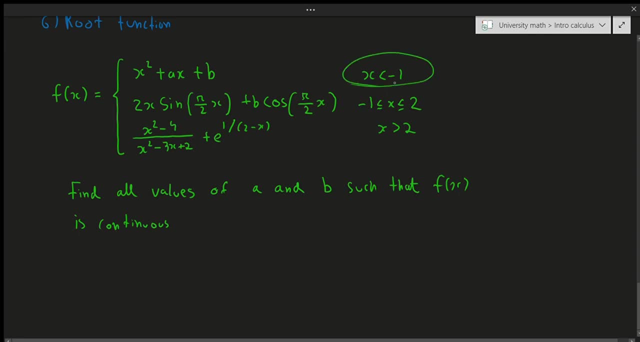 the limit as X approaches negative 1. as the limit as X approaches negative 1 of this function has to equal the value add negative 1, so let's go ahead and do that. so the limit, so let me just use a different color for this. so the limit as X approaches negative 1 of f of X equals f of negative 1. 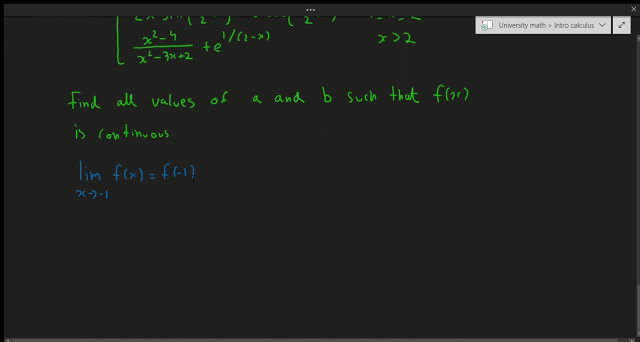 okay, Okay, so let's go ahead and do that. So, if I go ahead and do this, so let's, yeah. So in this situation, I can plug in negative one for this second one, because that's when the equal sign actually appears. 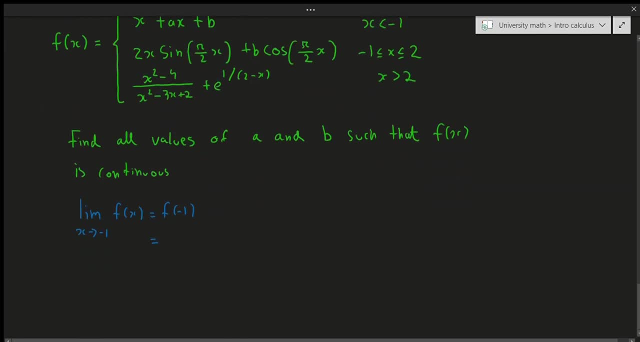 And then for this one I just cut the limit. So in this situation we've got to take the limit as x approaches negative one of. let's see it's going to be: x squared plus ax plus b is equal to two times negative one. sine of pi over two times negative one. 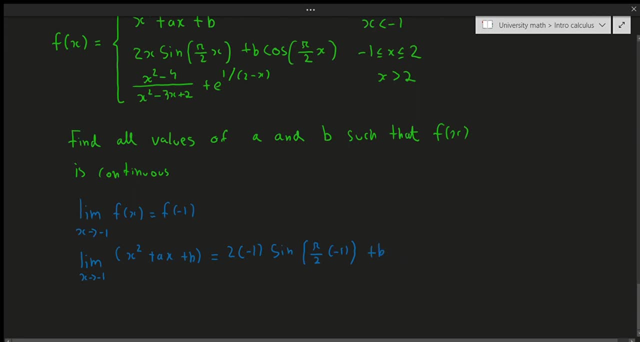 plus b cosine, Okay. so if you go ahead and simplify all of this, you're going to get- let's see, on the left-hand side you're going to get- negative one squared, minus a plus b. So that's going to be one: minus a plus b is equal to okay on this side. 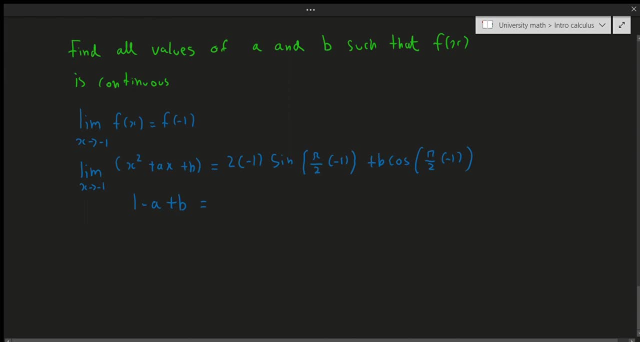 the cosine part is going to be zero. So you end up getting- let's see, that's going to be negative- two sine of b plus b, So that's going to be negative two sine of minus pi over two, So that's going to give you a two. 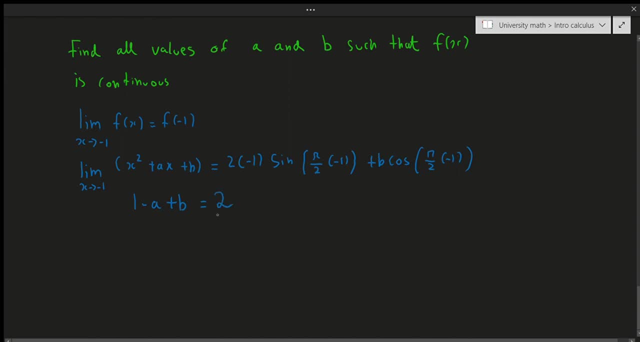 And then on this side, let's see: so you're going to get, if you simplify all of this, you're going to get b minus a equals one, So that's one system of equations. Okay, and then let's see the next one. 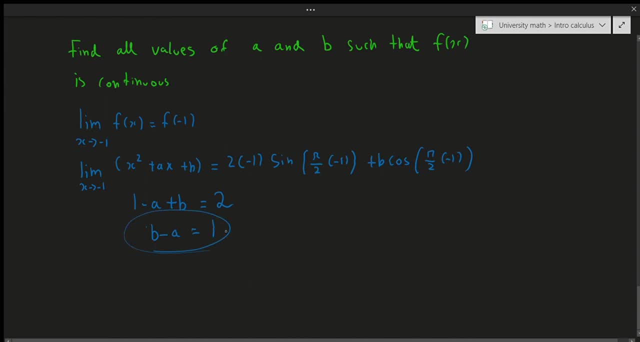 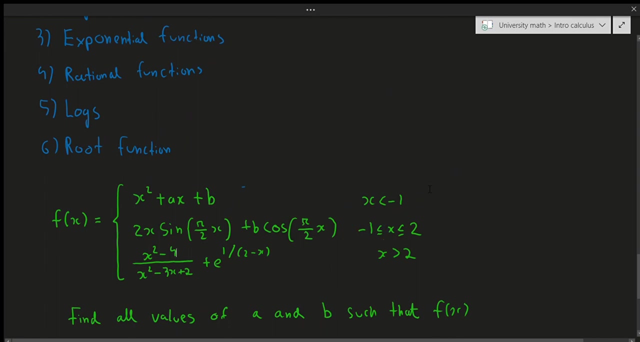 So we have now gotten one system of equations, So we need another set of equations To solve for a and b, So let's go ahead and do that. Okay, so we use the fact that it's going to be equal to negative one. 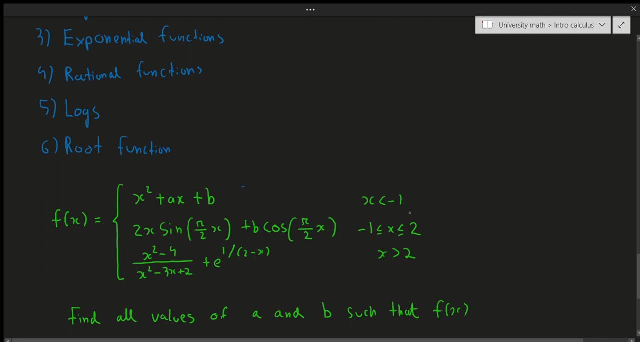 And then we can do the limit as well. And then for the second half we can do kind of the same thing: We're going to take the value as it's equal to two, And then we're going to check the limit as the function approaches two. 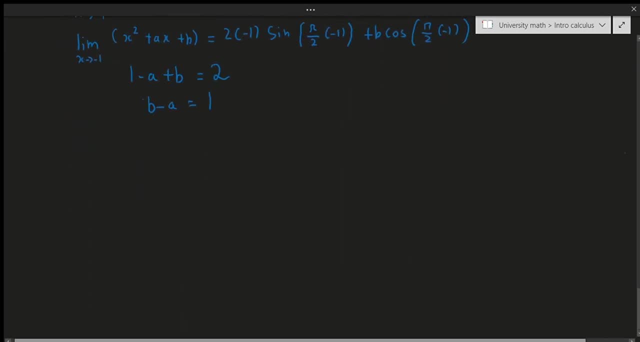 and see if those are equal, And then, using that same property, we can use it to get another system of equations. Okay, so let's go ahead and do that. So, in other words, the limit as x approaches two- Sorry, my pen is a little bit weird. all of a sudden, 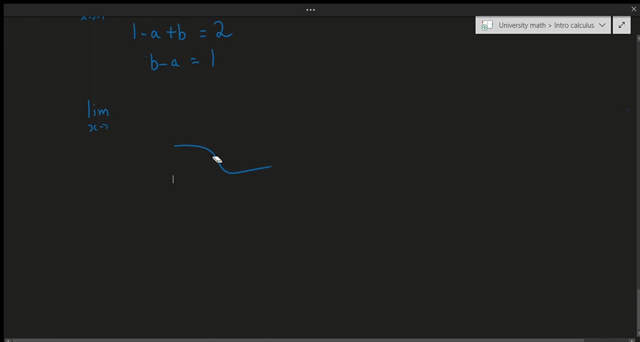 So the limit as x approaches two, There we go, Sorry about that. So the limit as x approaches two of f, of x must equal the value add to itself. Okay. so let's go ahead and do the right. Let's go ahead and do the right side first, because that's a little bit easier. 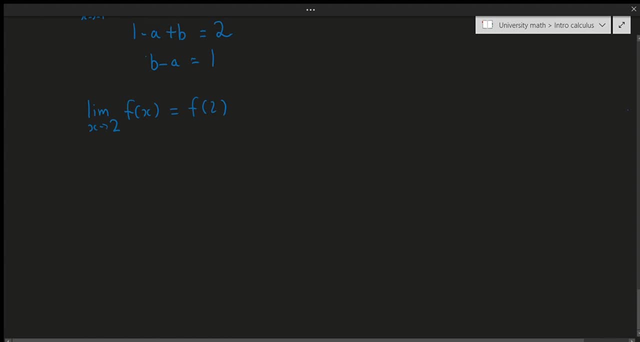 So if I were to plug in f of two, well, that's going to give me. well, let's see here. Okay, so what happens here? So in this situation, we have this kind of mess for two. So if we go ahead and do that, 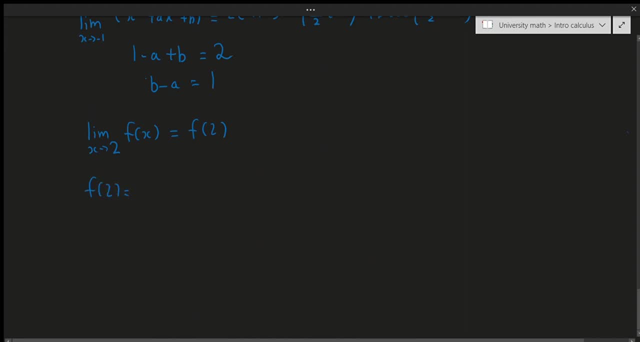 So f of two, that's equal to two times two, sine sine of pi over two times two, plus b cosine of pi over two times two, And if I go ahead and simplify this, we get four sine of pi. Well, that's zero. 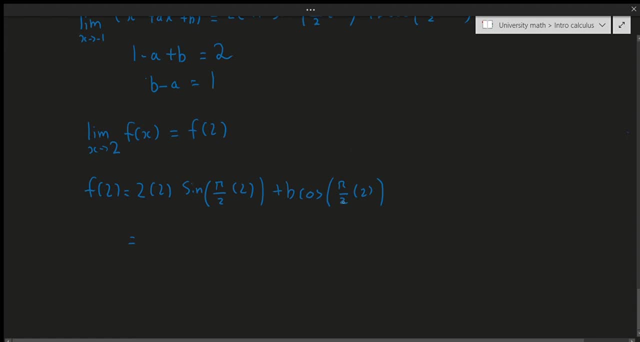 And then we get b cosine of pi over two times two. So that's going to be b times negative one or negative b, And then for the limit we got a. well, the limit is a little bit harder, So let's go ahead and do that separately. 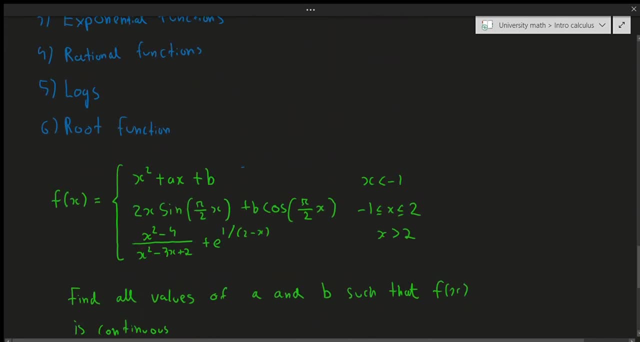 So we got to be a little bit careful here. For this one notice: we're taking the limit as x approaches two from the right. That distinction is going to be very important, because if we were to do it from the left, this limit would actually not be possible. 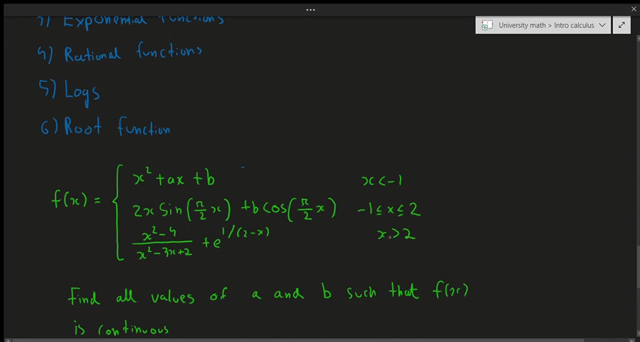 So let's be very careful about that. The reason it's approaching from the right is because x is bigger than two. So when the limit as x approaches two, when we do the limit as x approaches two, we have to do it from the right. 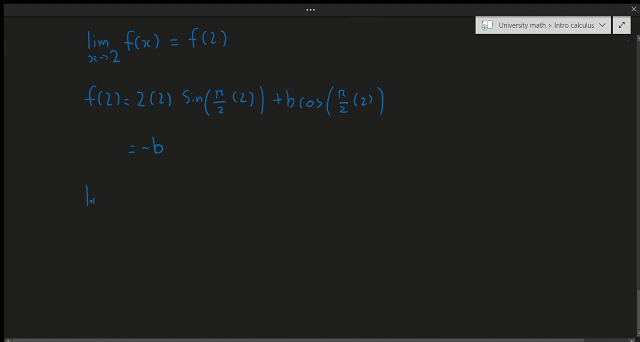 So let's go ahead and do that. So what happens when the? what happens for the limit? The limit as x approaches two from the right? okay, of f of x, let's go ahead and move that down. Okay, So that's going to be equal to the limit as x approaches two from the right. 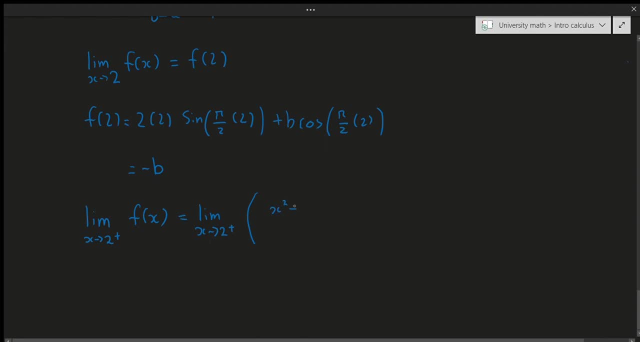 Let's see. So this one is going to be x squared minus four, divided by x squared minus three, x plus two plus e to the one over two minus x. Okay, So let's do this a little bit slowly. This one, this one, isn't so bad. 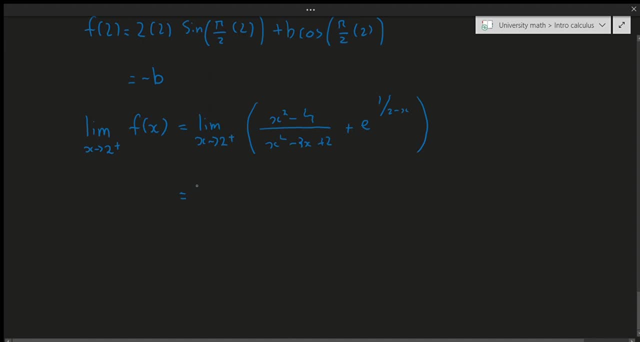 This can just be written as a factor, So we can use the limit properties where we can split this as the sum of two limits. and I know we can split it because the limits are going to exist. They have to, otherwise the function wouldn't be good to do this. 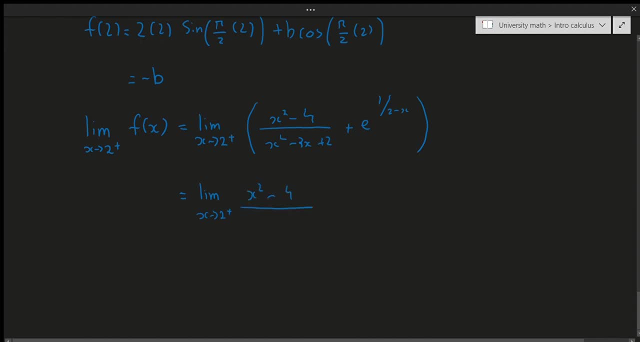 So let's go ahead and split this, So x squared over four, x squared minus four, sorry, over x squared minus three. x plus two plus. let's see the limit as x approaches two from the right of e to the one over two minus x. 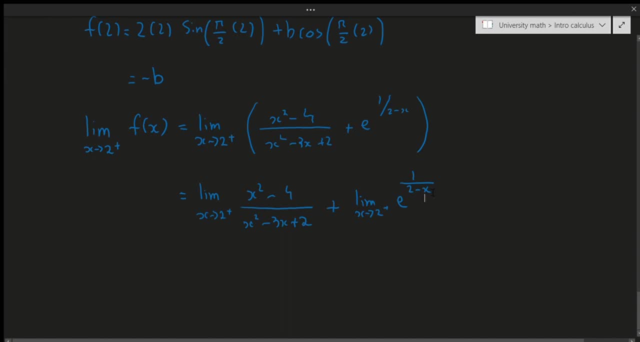 Okay. So let's go ahead and simplify. Let's simplify this a little bit more. Notice that this can be factored. So if I go ahead and factor this, we get the limit as x approaches two from the right. Uh, let's see that's going to be x plus two, x minus two. 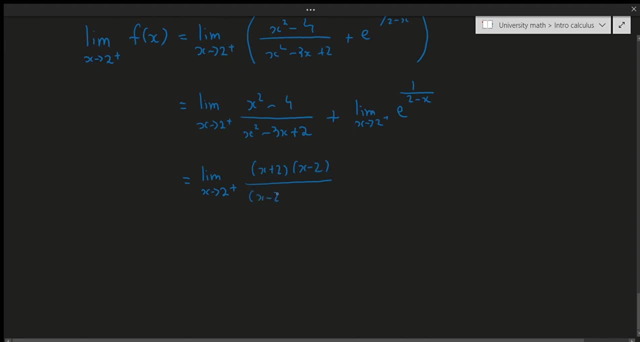 And then this bottom: that's going to be x minus two, That's going to be x minus one, And then, that's not too bad, We're going to leave you, we're going to leave this limit alone for a bit. Okay, now, conveniently, this cancels and then we can plug in a two. 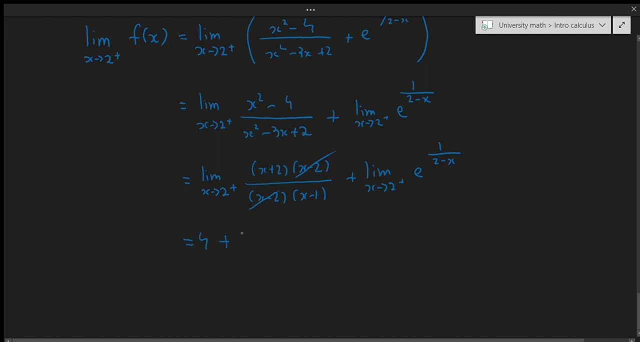 So that's going to give us four. and then we have to limit as x approaches, two from the right of e to the one over two minus x. So let's go ahead and write this down. Okay, Now what about this limit? This limit, we can't just plug in a two, because that would give us one over, well, zero. 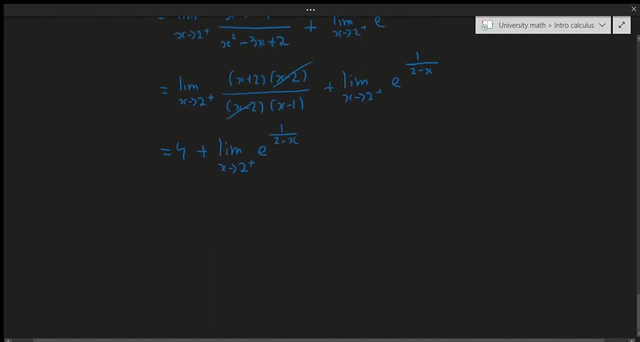 And that's undefined, But we got. but if you notice this, this is the limit as x approaches two from the right. So it's more like it's, for example, it's going from four to three and then it's going to two. 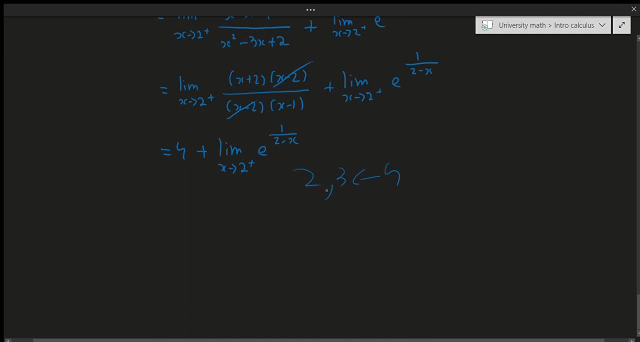 And then it's going to one. It's: oh sorry, there shouldn't be a one there, But the point is like it's going from a bigger number to two, It's not going from a smaller number to two, And that distinction is very important, because that's going to help us well a little bit later. 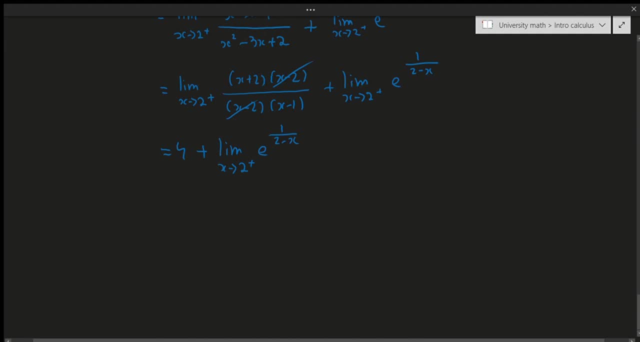 So suppose I plug in a number that's very, very close to two, but slightly larger than the two. So that's going to give us- let's see, that's going to give us- e to the power of. so I'm just going to do this on the side, using a different color. 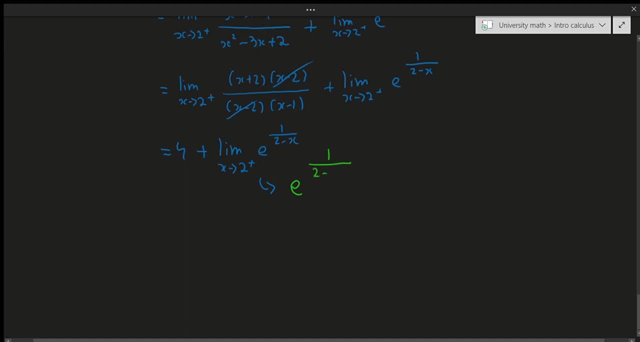 So that's going to give us e to the one over, two minus. let's pick a number that's just a little bit bigger than two, So 2.001.. Okay, Well, that's going to give me e over, sorry e to the power of. well, that's going to give me minus 0.001.. 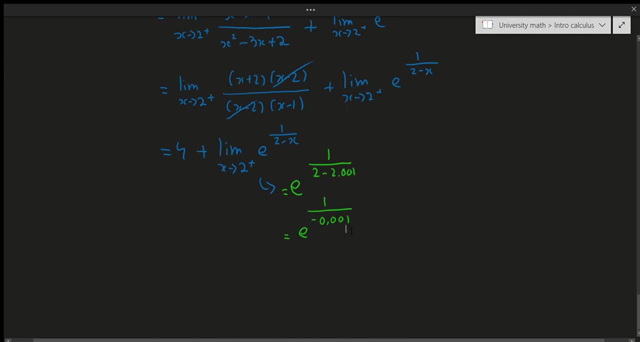 Okay, Okay. And then, of course, one over a really small number is very big, So that's going to give me e to the power of minus 1000.. And consequently, that's going to be e to the power of 1000. 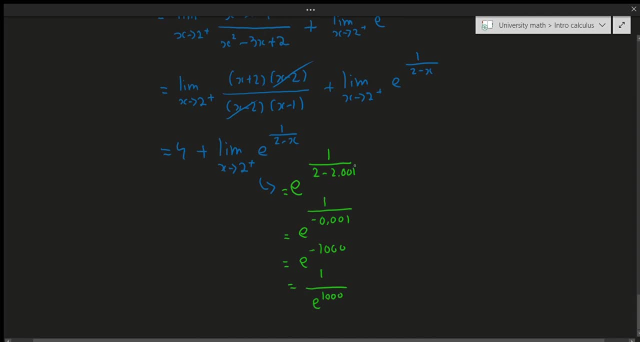 And that's going to be really small. But what if I make this even smaller, So like 2.000000, like all the way to zero and then one? That's going to be really small, But the point is, but the point I'm trying to make is that eventually, as this difference goes, 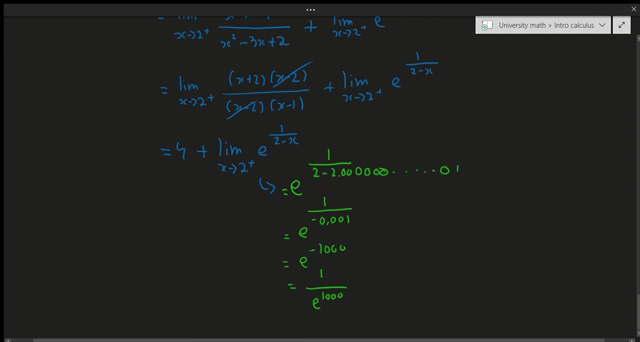 zero, that's eventually going to go to zero as well. So what I'm trying to say is the limit. as two x approaches two from the right, this difference is going to get so small that you're going to get a really small exponential. 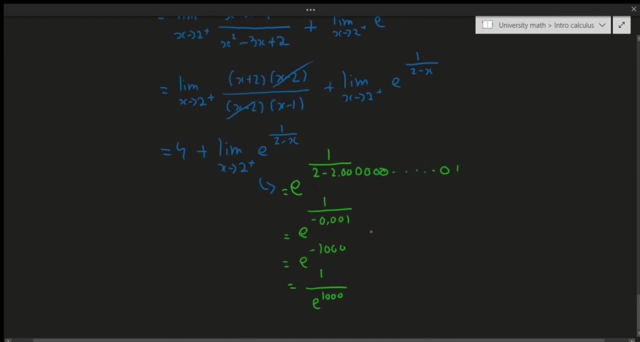 And eventually, as that limit gets closer and closer to zero, as in this limit, this difference, rather as it gets closer and closer to zero, this exponential, as a result, is going to eventually go to zero. So this limit is actually equal to zero. 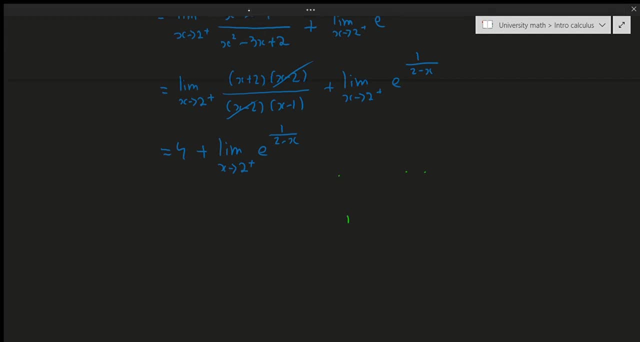 So that makes things very nice. So let's switch back to blue. So this limit, right there, is equal to zero. So we get four plus zero. And then, as we checked earlier, f of two was equal to minus b, So minus b is equal to four. 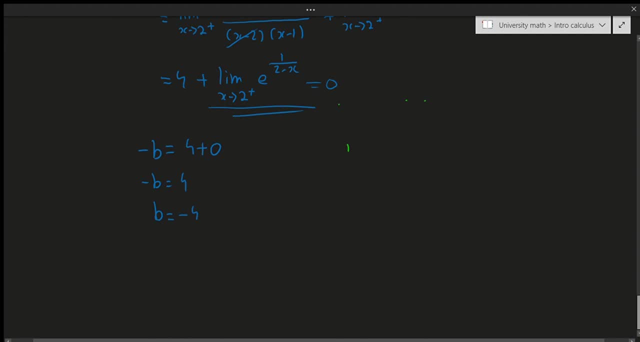 So consequently b equals negative four. Okay, so we're almost done. We also have this equation that b minus a equals one, So let's go ahead and write that down there. So b minus a equals one, and then negative four minus a equals one. 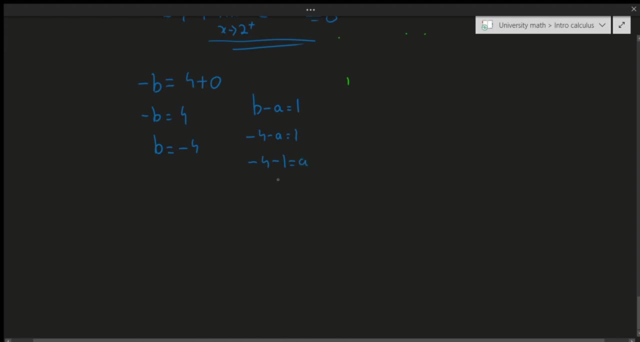 So minus four minus one equals a, and then minus five equals a. So there's that. So that wasn't so bad. Okay, so we're almost done now, And that's it. We are basically shown that for some. so for a equals negative five. 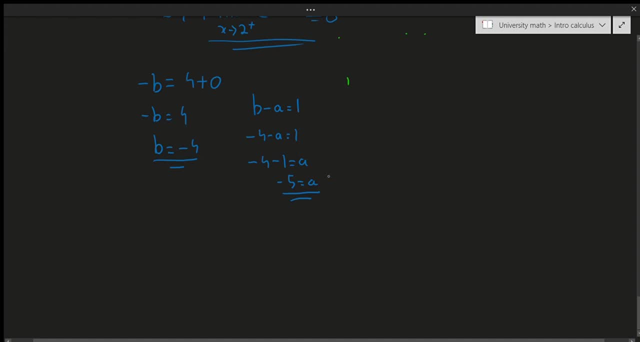 and b equals negative four. this function is continuous And that's it. So that basically takes care of continuity And I believe that covers everything you can talk about for the purposes of continuity, at least Probably just about anything you can cover for like an exam or something. 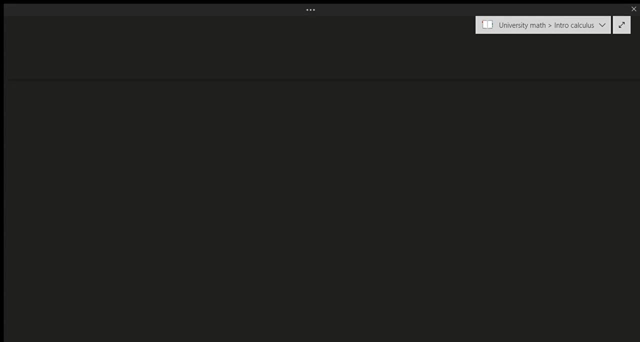 Okay, now let's talk about something new called the intermediate value theorem. So what is? so? that's a very simple theorem, So let's go ahead and write that down. So I'm going to use white for this one. So the intermediate value theorem. 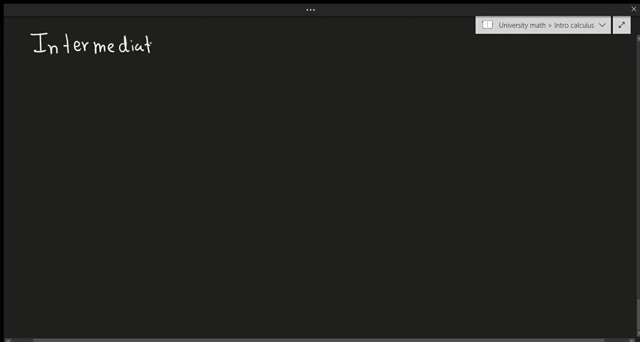 So intermediate value theorem, So sometimes it's called the IVT. Okay, so this theorem is very simple. There are a few caveats, but I will specify that as needed. So let's use blue And let's use a graph. 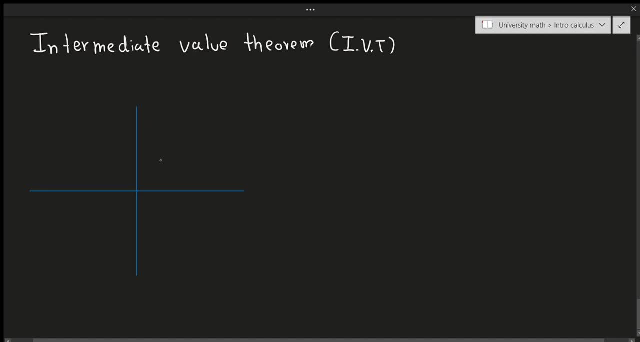 So suppose I have a continuous function on the closed interval from a to b. So here's my graph. So let's suppose we call that a, And then let's suppose we call that f of a, And suppose, furthermore, I call this b. 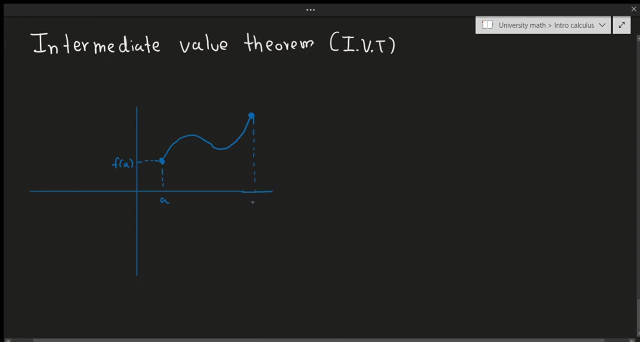 So let's go ahead and specify that. So let's suppose I call that b, And suppose I call this, And suppose I call this value. Sorry about that, It keeps erasing for some reason. So that's going to be f of b. 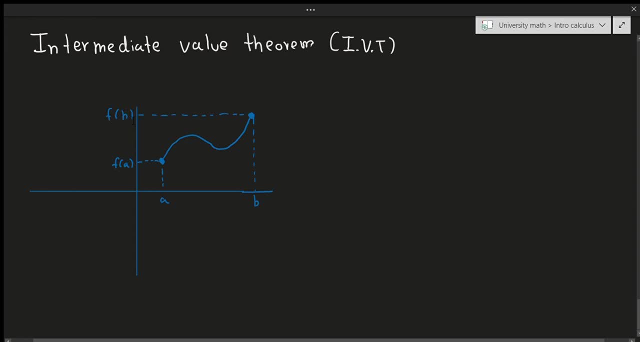 So the intermediate value theorem is very simple. It just says that between on the interval from f of on the closed interval a to b, there is a: y equals k, such that at some point x it's equal to the value. Now again, that might seem a little bit complicated. 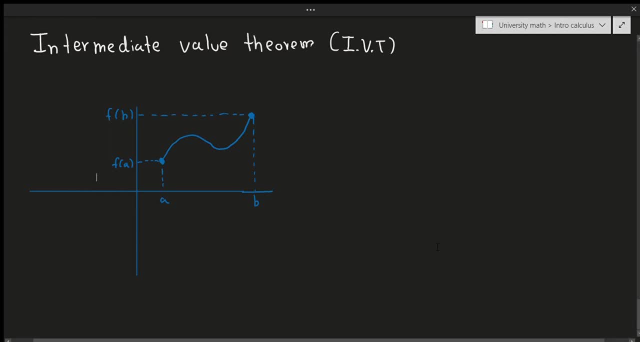 So let's kind of digest that a little bit On the closed interval a to b. so on the closed interval a to b and let n okay. so let's be really clear about this. This has to be a closed interval. 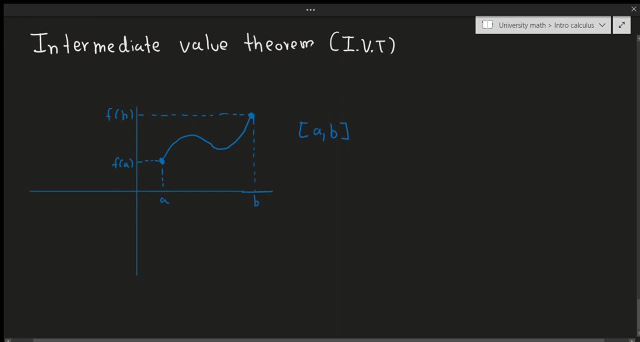 Next, let n be any number between f of a and f of b, So let's call this value n, right there? Okay, There exists a number on the open interval a to b, such that f of f of c equals n. So what does that mean? 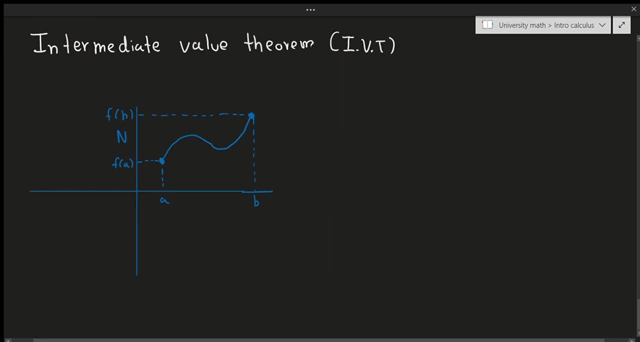 So let's again digest. let's just digest this very carefully. On the closed interval from a to b, there is a number n, such that f of c equals n. What does that mean? I'm basically saying that between the closed interval a to b 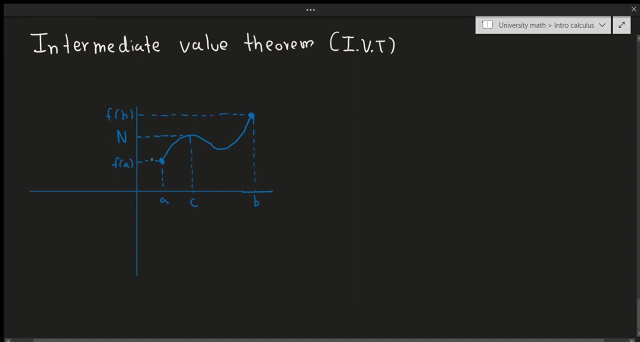 every number in between f of a and f of b has to exist If the function is, if the function is continuous. Now, that's kind of obvious if you think about it. If a function is, you know, continuous, so if it's, let's say, it's a random kind of graph like this: 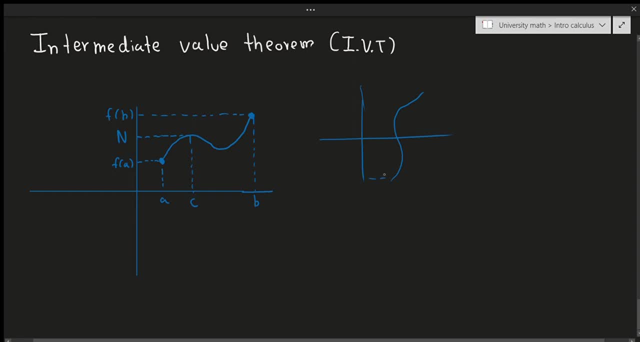 and this right there is f of a, and this right there up there, let's call, let's call this f of b and let's say that this right there is a and let's say that this is b. right there. 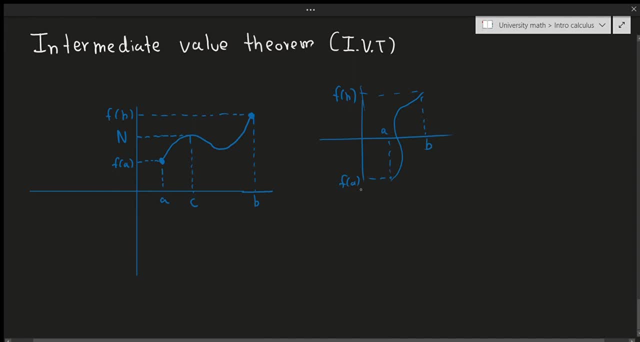 Well, if I'm saying the function is continuous from a to b, so that would be, and that would mean that every value between f of a and f of b has to exist. So, for example, this value has to exist, this value has to exist. this value has to exist. 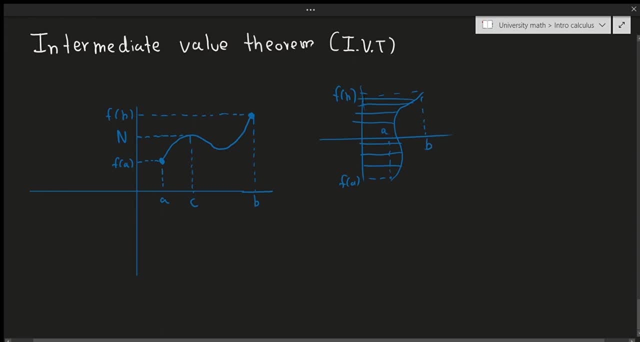 this one has to exist, this one, this one, this one, every value between f of a and f of b, they all have to exist. So it's kind of the same idea here. So if I call that n, for example, sorry about that, the screen just jumped. 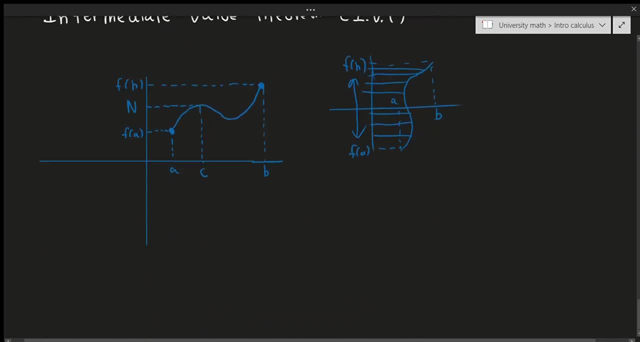 So if I call that n, every value in between f of a and f of b has to exist. So, for example, n1 has to exist. that's this point. right there, n2 has to exist. right there, every value in between has to exist. 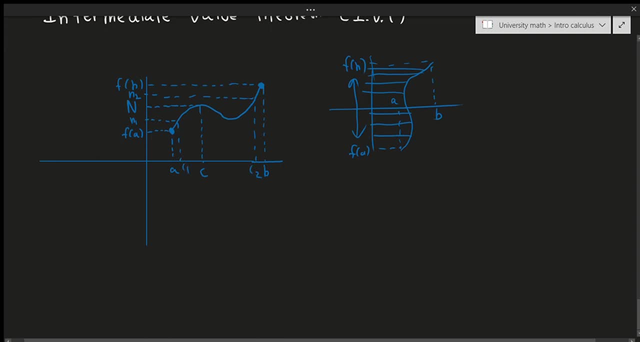 And that should kind of make sense. So let's call it c1, c2.. So I'm just saying that for every value between f of a and f of b, the y values in between all have to exist, if the function is continuous, for some corresponding x value. 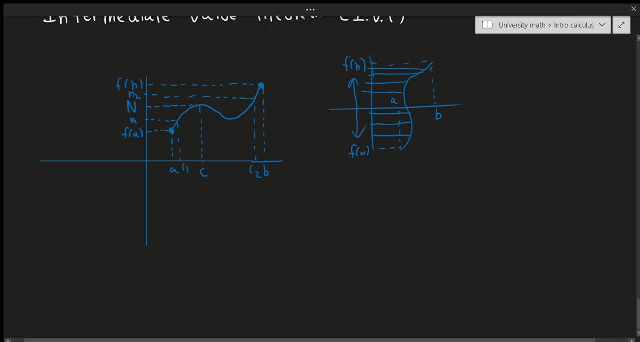 So, for example, between f of a and f of b: f of c equals n, f of c1,. let me just fix that c1 is equal to n1.. f of c2 equals n2.. So every value in between f of a and f of b have to exist for some corresponding x value. 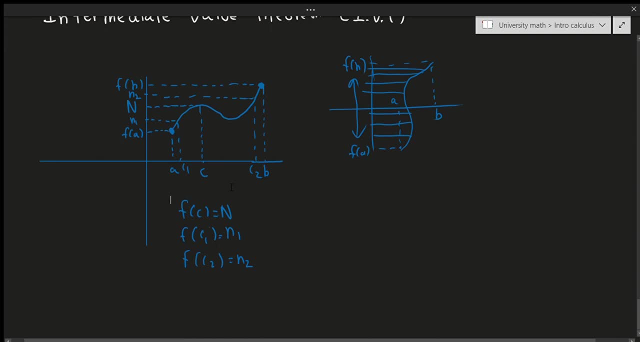 And now you might be asking: well, how is this useful? Well, the reason that this is useful is because it lets us do things that would have otherwise been really difficult. you might be asking what I mean by that. Let's just take a look at some really quick examples. 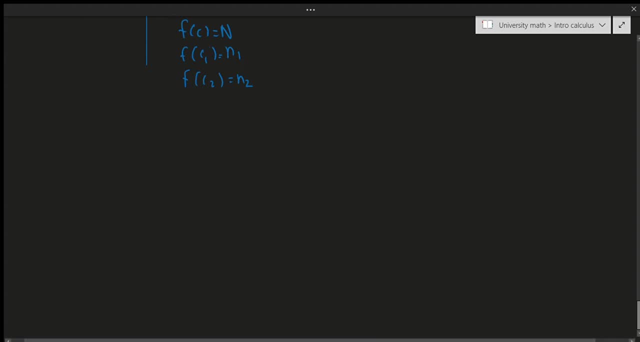 to kind of demonstrate my point here. So here's a very quick example. So show that there is a root of the equation: 4x cubed minus 6x squared plus 3x minus 2 equals 0.. So basically I'm trying to show that there is at least one root. 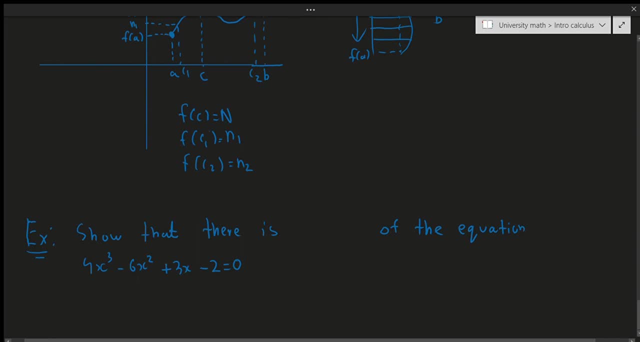 or I should probably specify that. show that there is at least a root, at least one root. Let me just fix that. So at least one root, One root to the equation. Okay, Show there's at least one root to the equation. 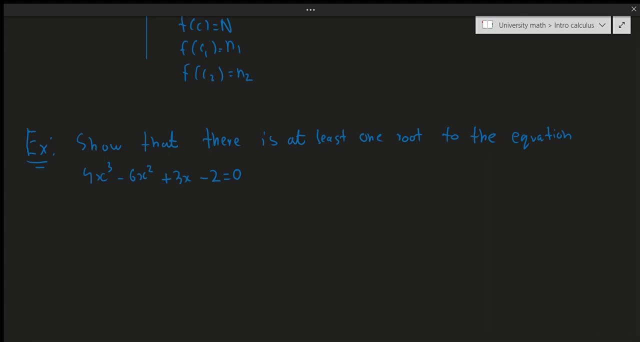 4x cubed minus 6x squared, plus 3x minus 2, equals 0.. So by root- I mean the root of an algebraic equation- just means that it intersects the x-axis. So basically there's a solution to this equation. 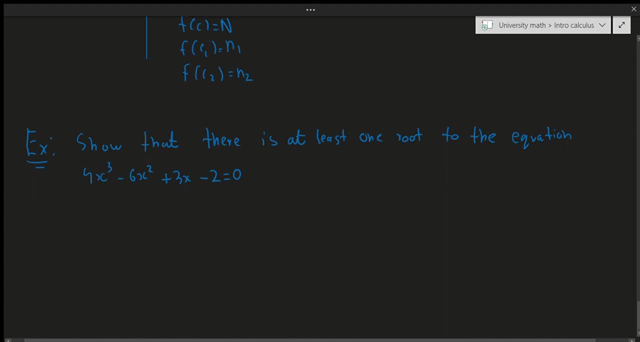 There could be more, but the point is I'm trying to show there's at least one. So how do I do that? Well, according to the intermediate value theorem, I have to show. every value between f of a and f of b have to exist. 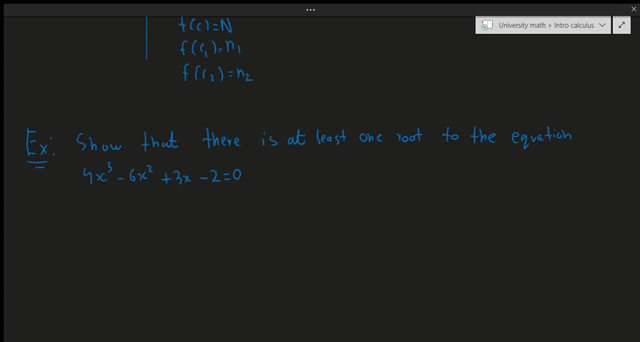 for some corresponding value for x. So what does that mean? How does that help us with this kind of question right here? Well, this is clearly a polynomial. So let's define f of x as 4x cubed minus 6x squared. 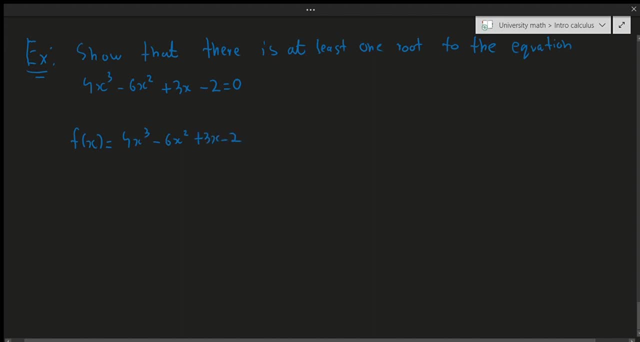 Plus 3x minus 2.. Okay, That would mean that if I could show that this is negative at some point and that this is positive at some point, because that's a continuous function, it has to go from negative to positive And if that's the case, it must have crossed the x-axis. 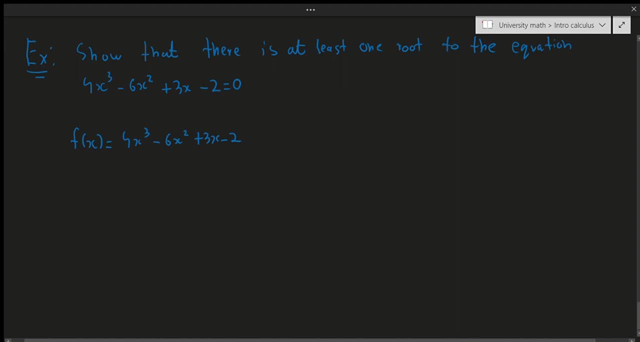 So what does that mean? That might seem a little bit confusing, So let's just kind of think about this for a second. So let's just randomly guess some values. That might seem a bit absurd at this point, But just bear with me. 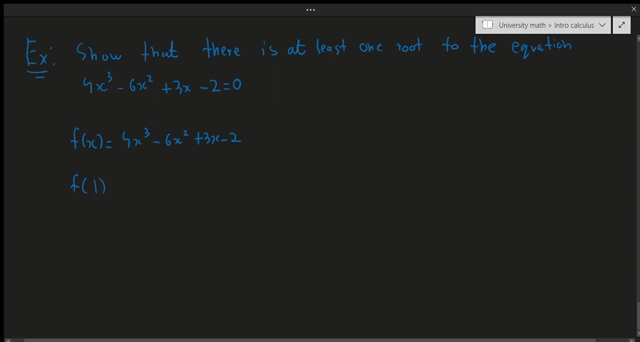 So suppose I tell you that f of 1 is something. So if I go ahead and plug it in, you'll get that f of 1 equals negative 1.. So let's make that a bit clearer. So f of 1, that's equal to negative 1.. 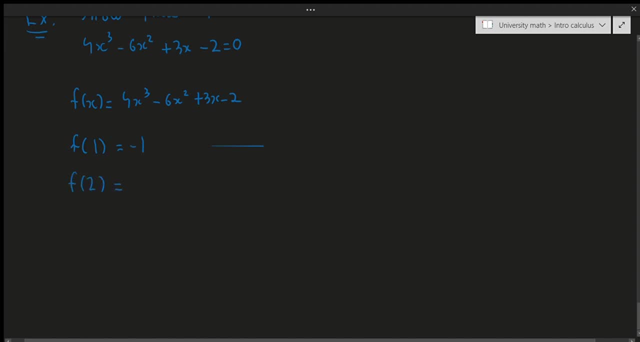 So, furthermore, suppose I tell you what f of 2 is. So let's go ahead and plug that in, And if you plug it in, you'll get 12.. Okay, So let's go ahead and kind of draw this a little bit. 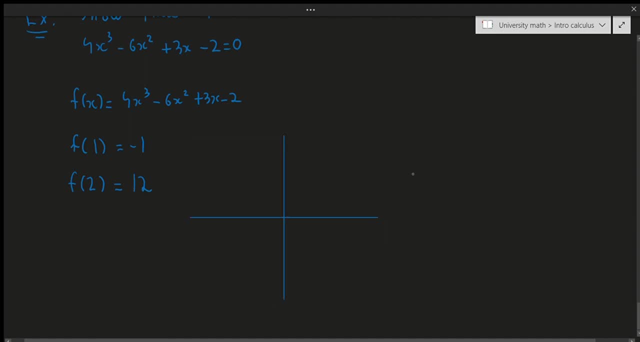 Now I must emphasize- Okay, I must emphasize- that I don't know what this graph looks like, But I do know that f of 1 equals negative 1. So let's go ahead and draw that, So that's like here. 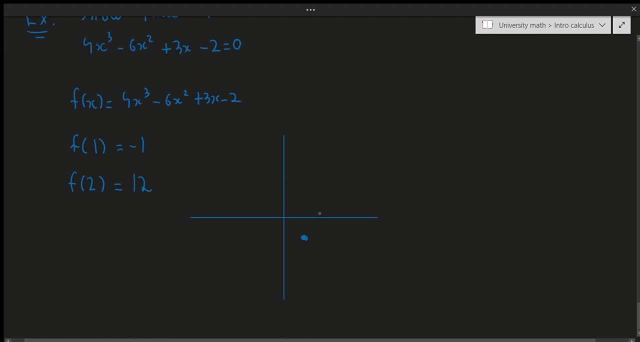 And I know that f of 2 equals 12.. So that's like about here And this is a cubic. I don't know what the like. generally a cubic looks like this, But I don't know what a shape looks like. 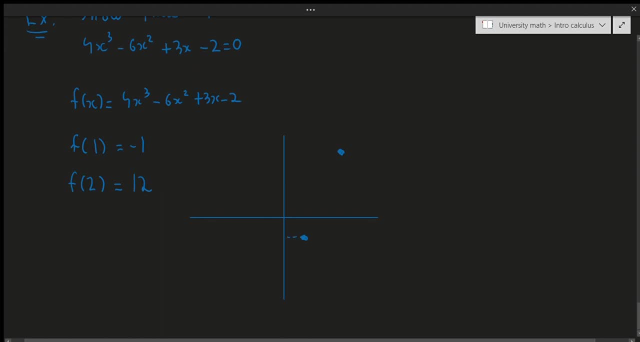 But I do know that this point right there. So that's: let's see, that's 1.. That's f of 1.. And then- So let's make that really clear- So that's 1.. And then this point right there. 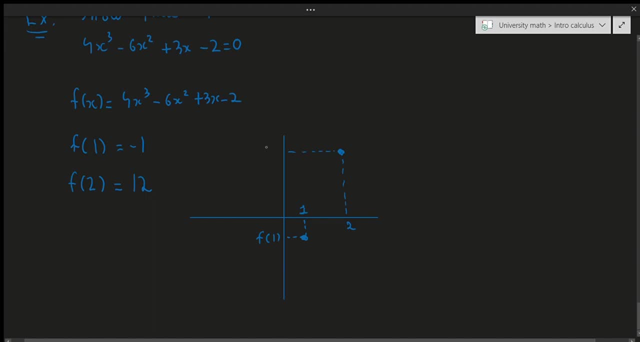 That's a 2. And that's 12.. Okay, I know that because this is a continuous function Because, as I mentioned way back here, Polynomials are always continuous. So I know that this is a continuous function And I know that. 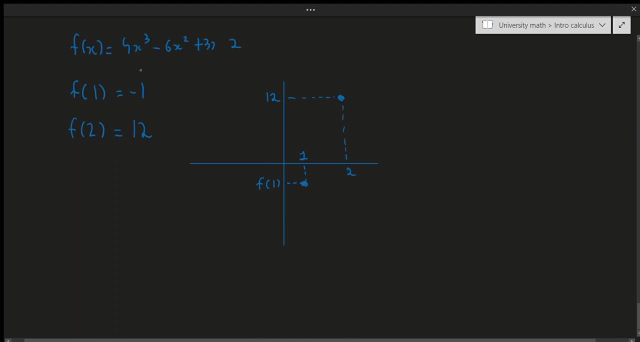 I know it's continuous on the interval from 1 to 2.. So it's continuous on the closed interval 1 to 2.. So that means I must have So in order to reach from f equals f of 1 to f of 2.. 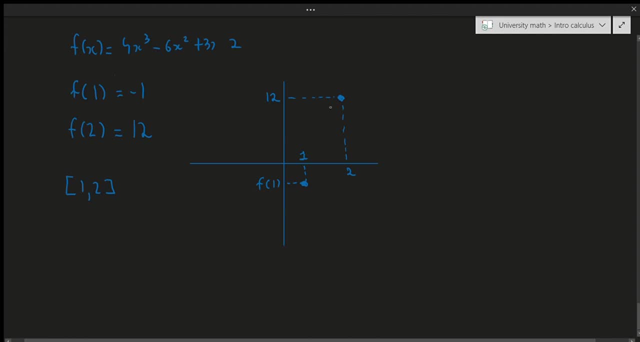 I must have crossed the x-axis. Now I don't know where I crossed the x-axis, But I know I must have crossed it at some point, Because it's a continuous function. I can't just, I can't just suddenly jump like that. 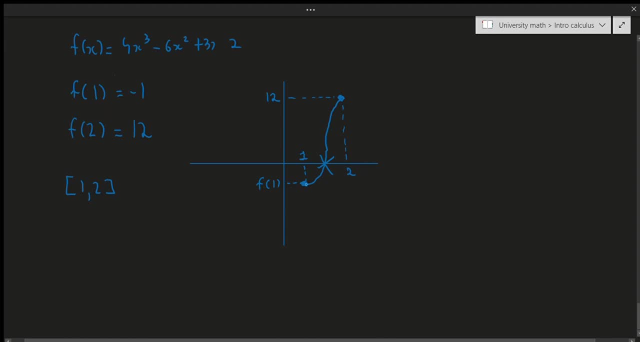 Like that doesn't make any sense. So in order to cross from negative 1.. So let me just really emphasize that to be clear, Just to be consistent. So that's f of 2. And that's 12.. So in order to go from y equals negative 1 to y equals 12.. 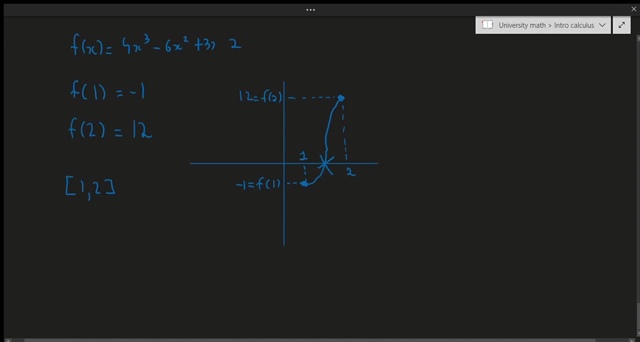 I must have crossed the x-axis Because it's a continuous function And, according to the intermediate value theorem, If the function is continuous on the closed interval from a to b, I must. Every value in between must exist. So in order to get from negative 1 to 12.. 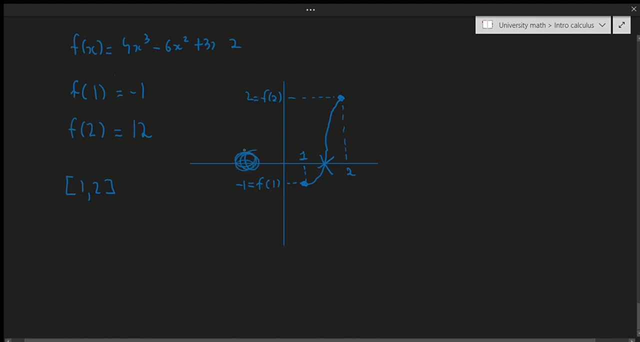 I must have crossed 0. I must have- Like that should be common sense- And because I crossed 0. There is an x equals c, Such that f of c equals 0. I don't know what that c value is. 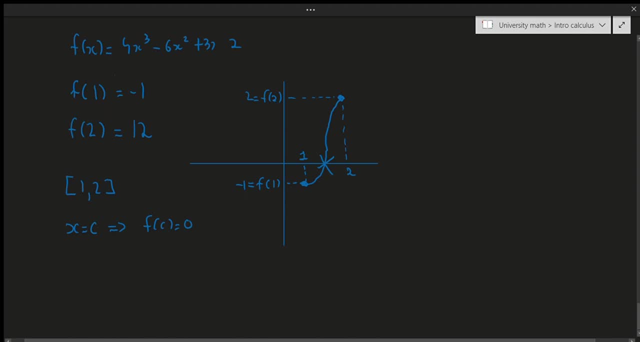 Like I don't know where it exists or whatever, But I know that I must have crossed it. So hopefully that makes some sense. And because I crossed the x-axis, I know there's at least one root. So therefore, By i b t.